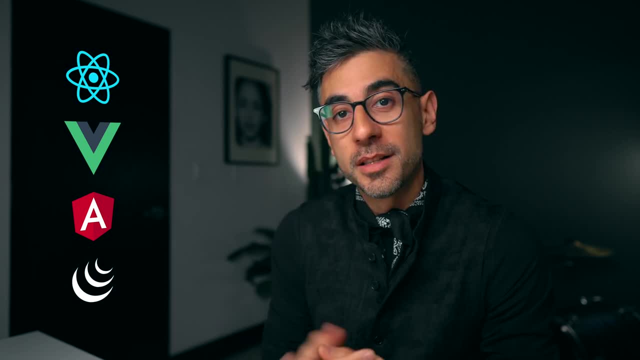 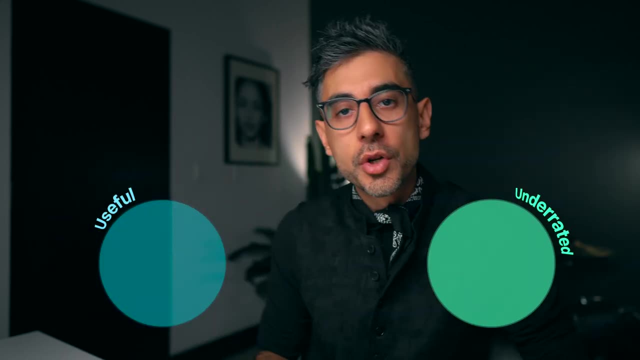 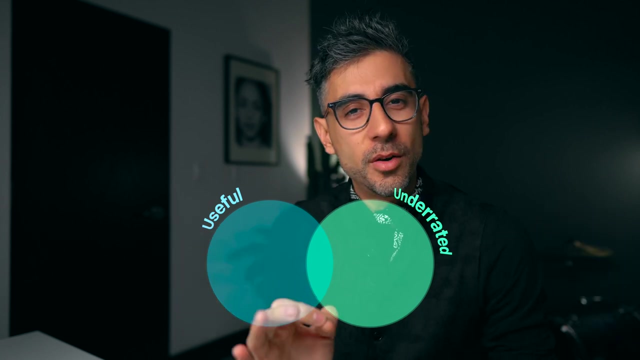 for that matter, they all use the same thing under the hood, which is eventually the almighty DOM API. If you take the most useful JavaScript APIs and then take the most underrated and understudied JavaScript APIs and overlap them into a Venn diagram, what you get at the center? 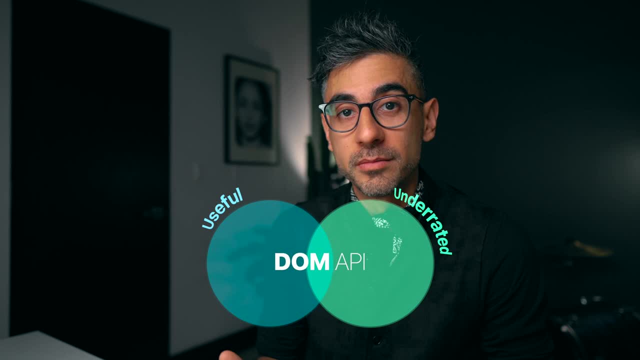 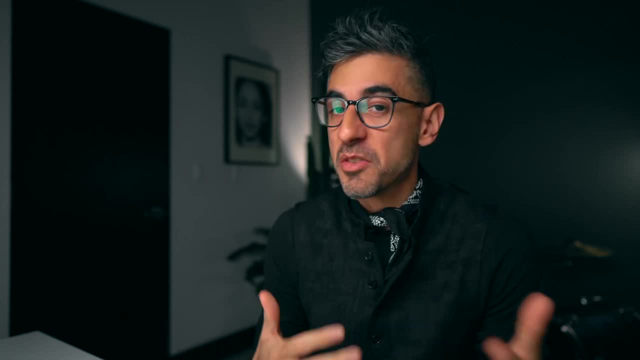 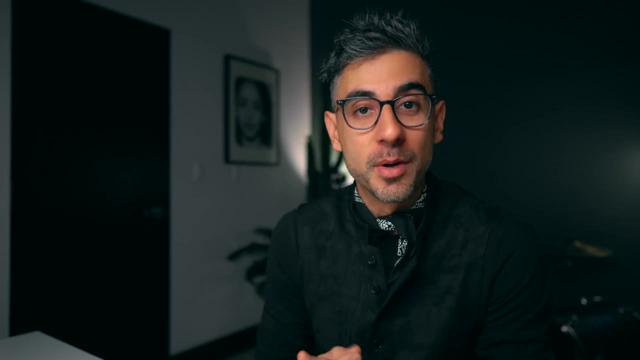 not directly. i didn't get exposed to it until maybe sixth or seventh year into my javascript career. so today we're going to mess around with the dom using a native browser api and obviously we're going to do it with pure javascript, no libraries, no frameworks, just you and me and the 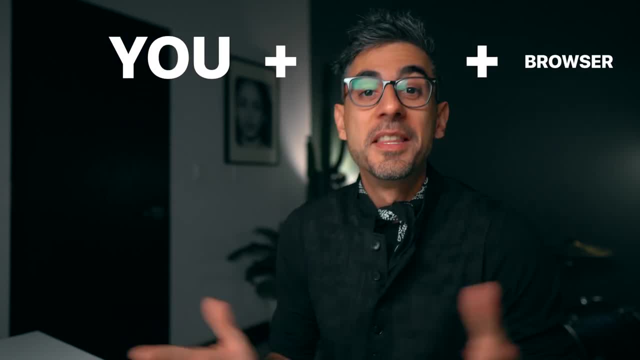 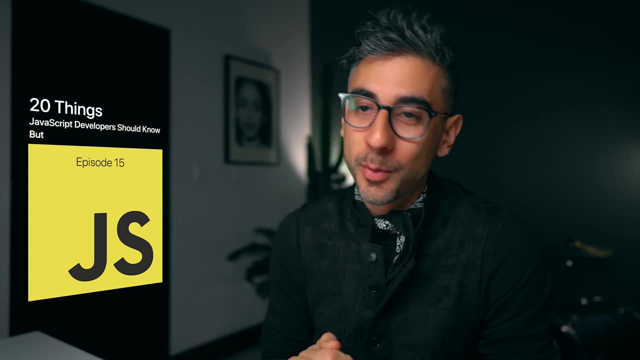 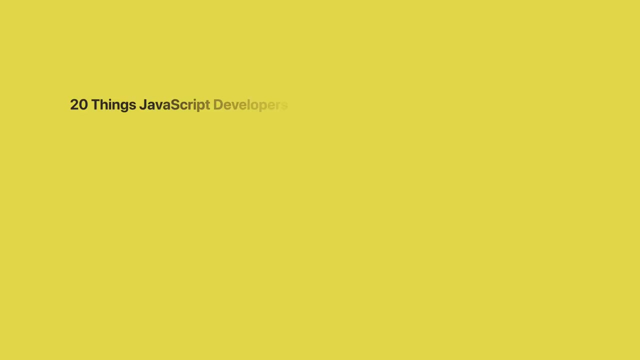 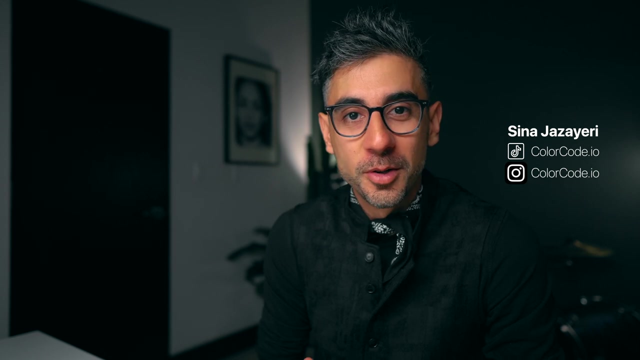 browser. we're going to make a to-do app with about 10 lines of code. this is episode 15 of this 20 part series. i'm calling 20 things javascript developers should know, but probably don't, as the one and only dummy. let's go hello. i've been gone a while. i know i missed you too. i got a bunch. 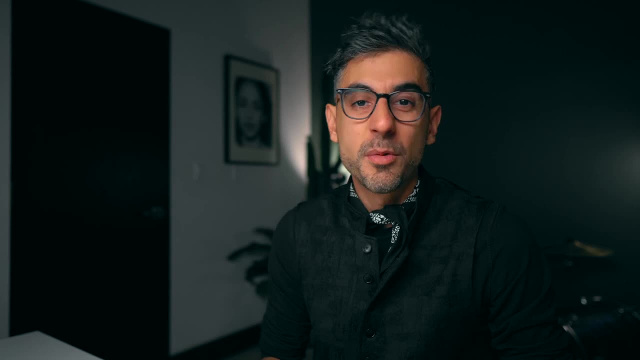 of comments asking where i was and if i was okay. i'm okay. i was mostly gone because of this. let's begin. if you've never directly worked with the dom, you should, and today is your chance. the dom api is part of a large list called the web apis that lets you do pretty much anything. 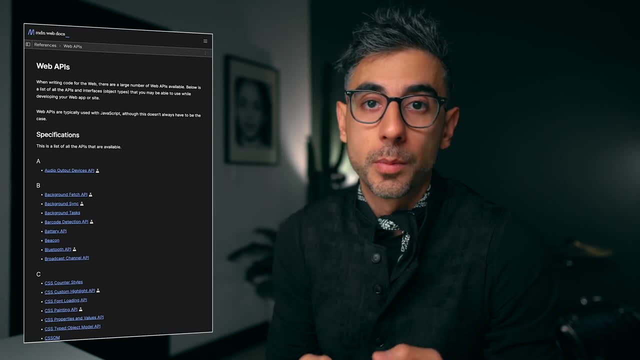 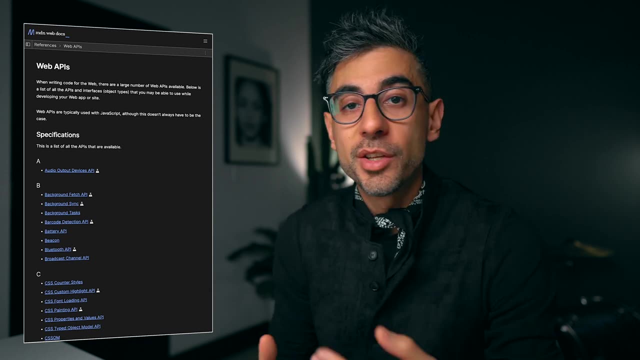 you want natively in the browser, without using a third-party library. and before we go any further for all of today, let me be clear. i'm not saying third-party libraries are bad. just like you, i use them every day at my work. all sorts of businesses and developers around. 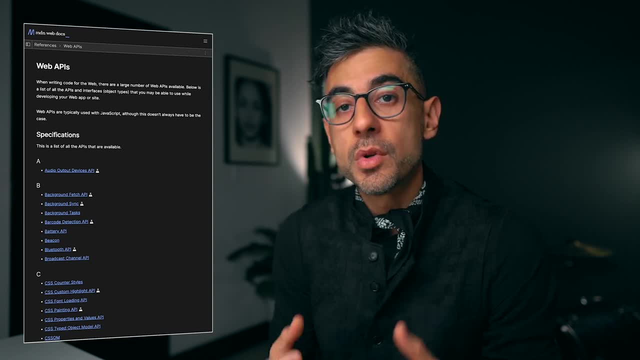 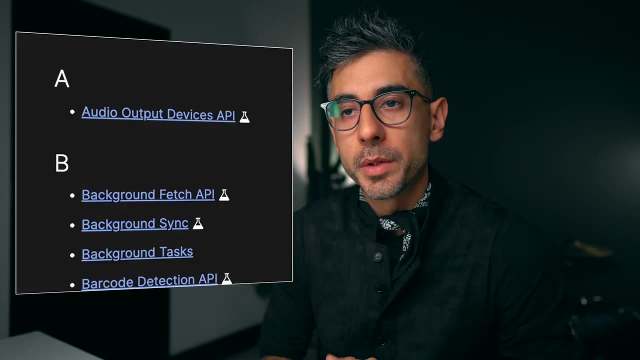 the world depend on them to do their day-to-day job, but the thing that most developers don't know, and they're not taught really, is how much you can do just using native browser apis. here's a list of all the web apis, including audio, battery, bluetooth, canvas. 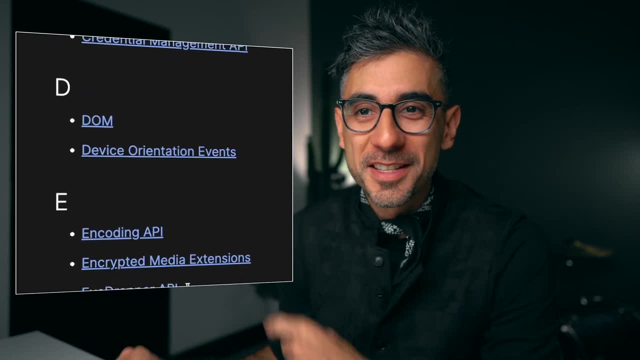 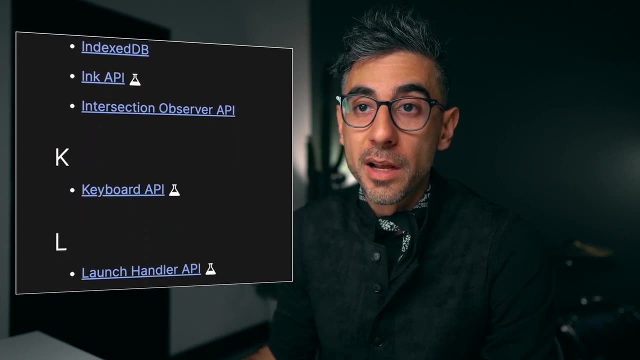 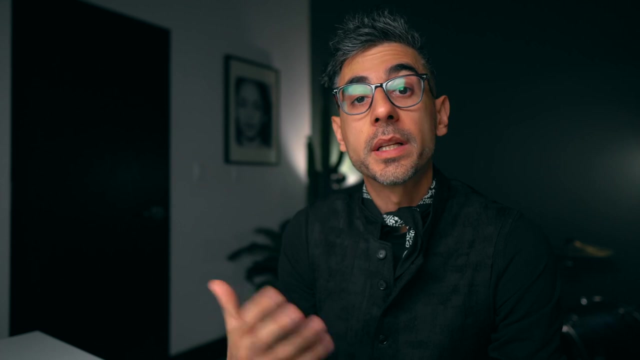 clipboard console cookies, dom. there it is. there's dom. uh, there's fetch api that i covered in the last episode and so many other things. you name it, it's there. a lot of these here are relatively new, but the dom was one of the first to get standardized and then really quickly it got. 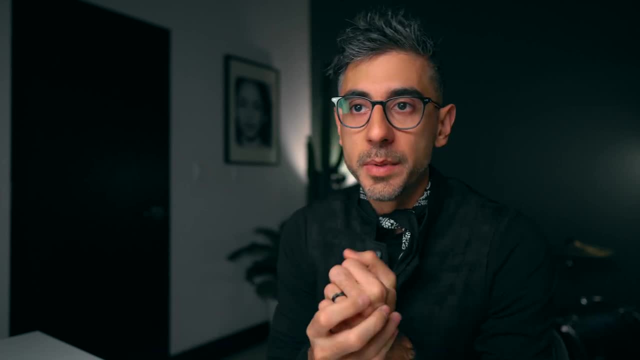 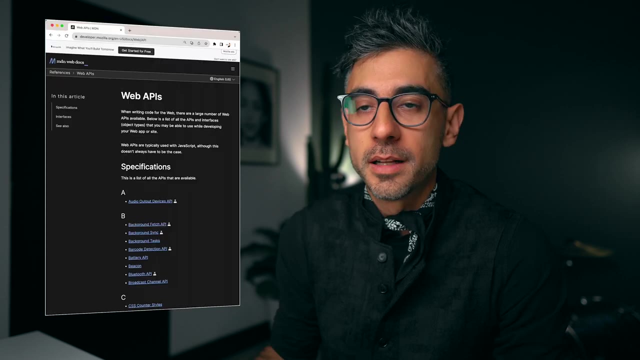 implemented into pretty much every browser. for us to understand the dom api first, we need to understand what the dom is. it's this, this whole shebang. you probably recognize it from your dev console when you right click on an element and say: in the bottom right corner of your browser, you'll see a list of all the web apis that you can use. 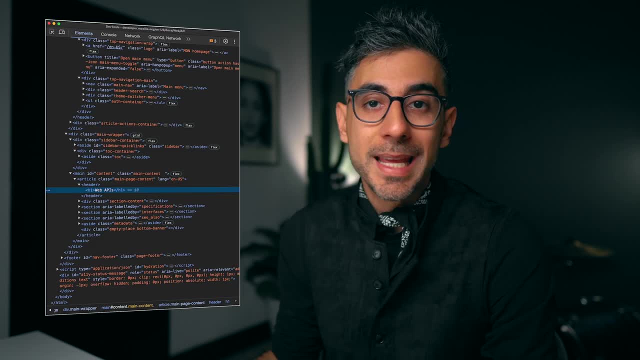 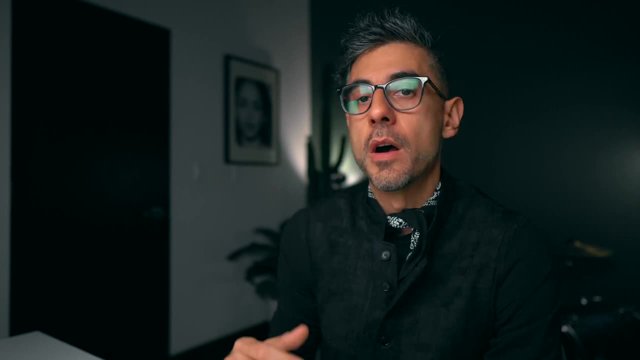 right click on an element and say: in the bottom right corner, you'll see a list of all the web apis that you can use. inspect element. this whole tree of html nodes is the dom and it's short for document object model. forget the name, it sucks, it's the pure data representation. 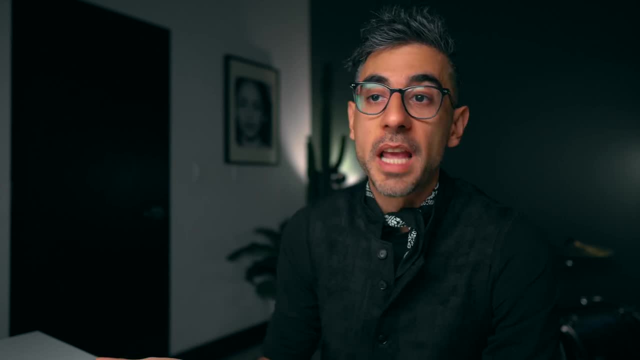 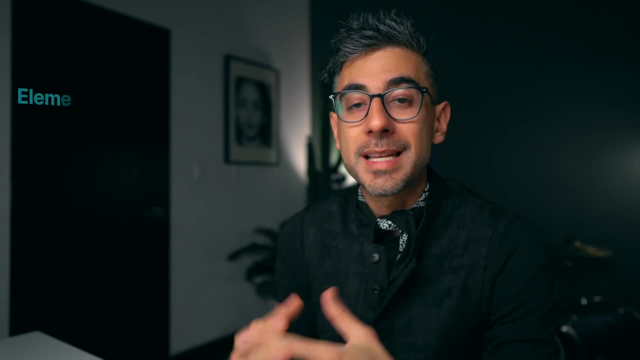 of what you see rendered in the browser. so now, what's the dom api? it's the api that allows you to access all of this stuff, all these elements, directly through code, javascript. it lets you find your elements, access their contents, their attributes, add event listeners, create new elements. 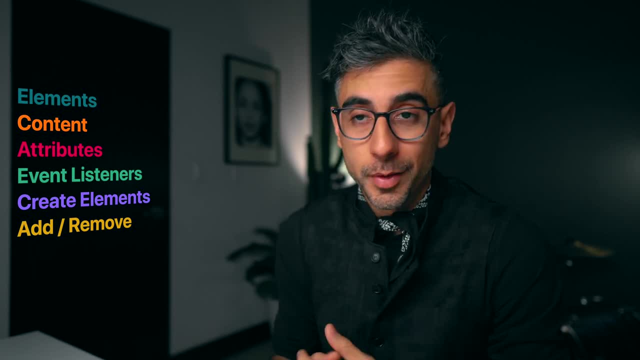 and add them to the dom or remove them from the dom and a lot of other crazy. that gives you total control over the page, aka the document. actually, you can clone react's source code from github- react dom that is- and search for some of the functions i'm going to show you today and see. 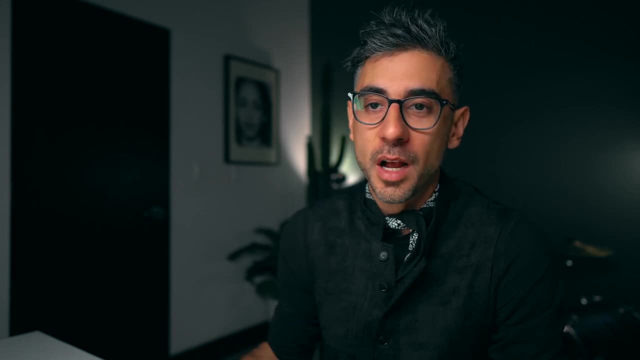 how frequently they're used. it's pretty wild. it's all eventually done through the dom api, because it's the most common and, from what i understand, the only entry point into the document. i think even webassembly has to call javascript to access the dom. okay, so today we're going to look at how to. 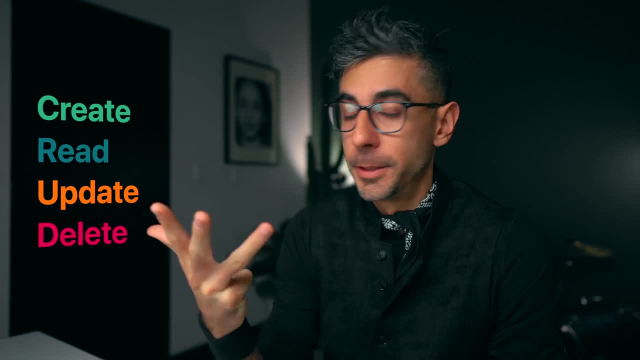 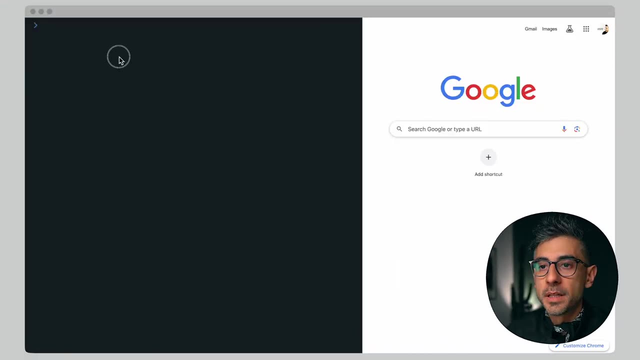 create, read, update, delete crud, and we're going to use, obviously, javascript. no libraries, just you, me and the browser. okay, open up your browser, open the dev tools and we can get started. so the dom has a bunch of what's called interfaces. we're going to use the document interface as our entry points through. 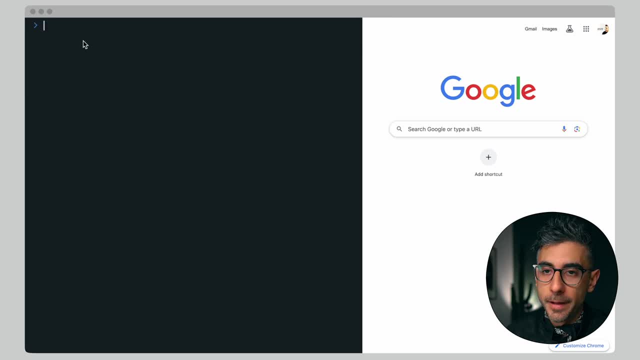 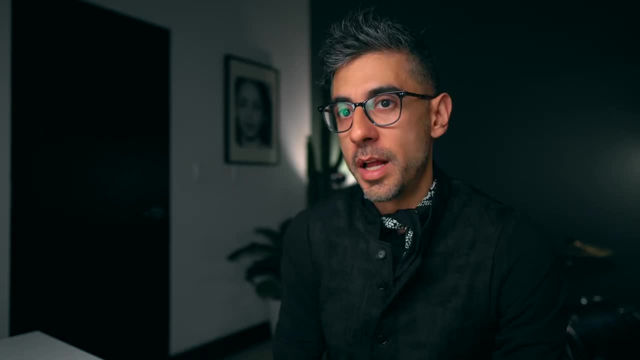 that we'll get to other interfaces, like elements and events and so on and so forth. and remember, what we're talking about today is within the context of the browser. last thing before we start writing code: anything i show you today is for your knowledge and demonstration purposes. 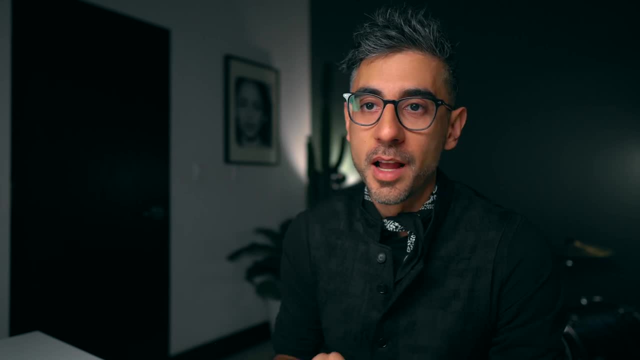 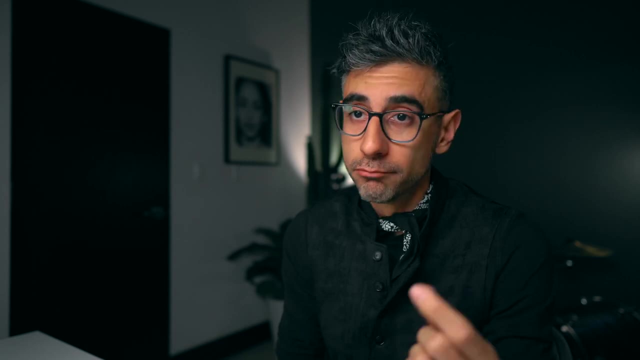 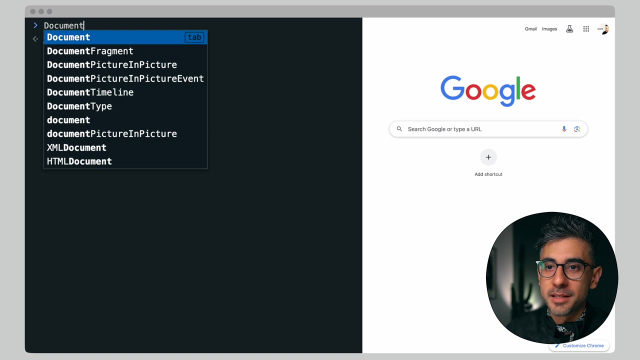 does not mean you should do this in production code. i'll be doing a lot of real-time stuff just in the console. it's just to show you what you can do with these commands. okay, okay, and with that, to the browser shrink. all right, we're going to start with an object called document. uh, actually. 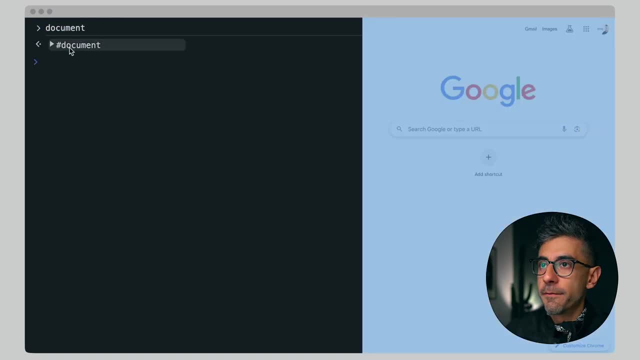 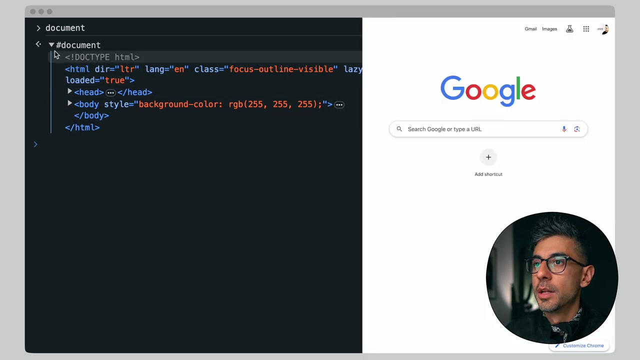 it's lowercase document. look at that. it gets highlighted. if i hover over it it seems to be the entirety of my page. if i click this arrow thingy it opens up. so chrome tries to be really cool and actually render the the whole inspect element kind of view for us here. 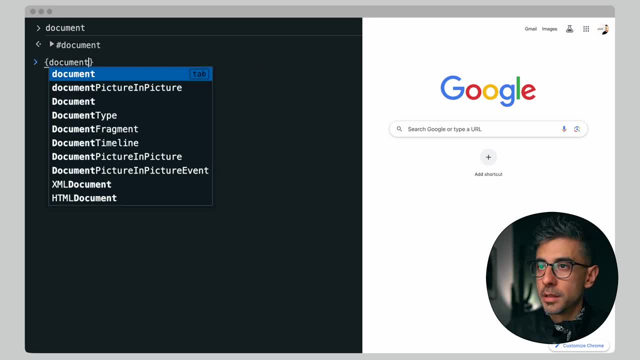 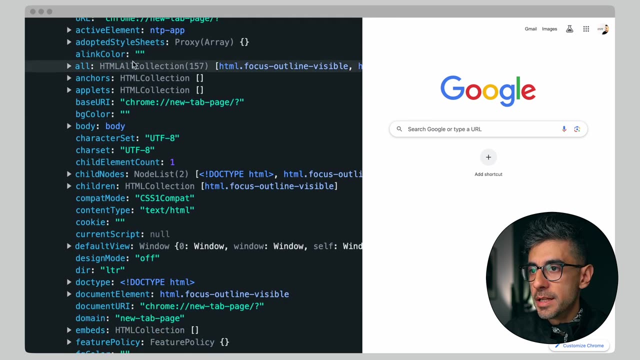 so what i'm going to do is i'm going to put this in an object like that, which is short for this document document, and when i press enter now i can see the object. okay, so let's go through the object. it has a lot of properties and methods. so what are some of these properties is? first of all, i have 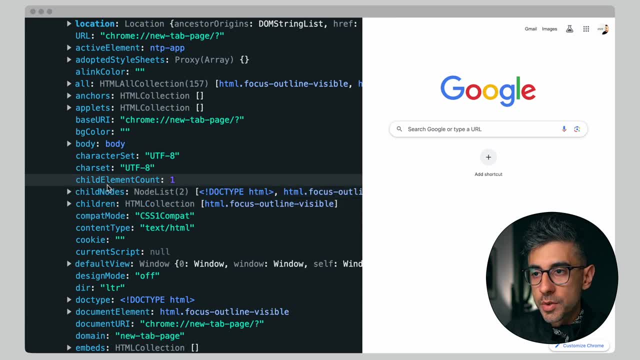 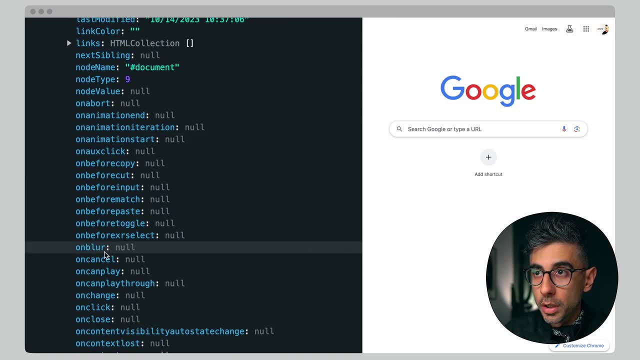 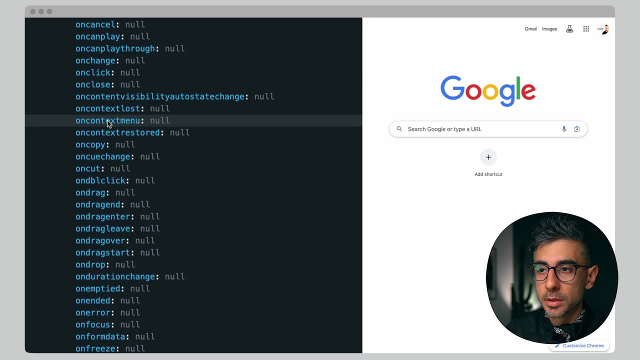 url. i have children, child nodes. we'll get to all of this i have. let's see. let's look at some of the methods on on blur, on click, these are interesting, okay. so on click, what is that? on double click, dbl click, there's a lot here, right? so clearly, document is an object that i can access and use its. 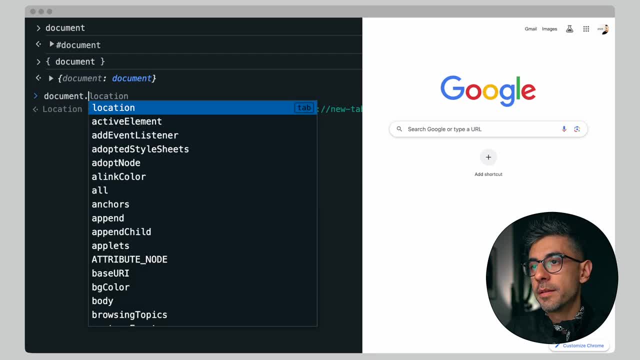 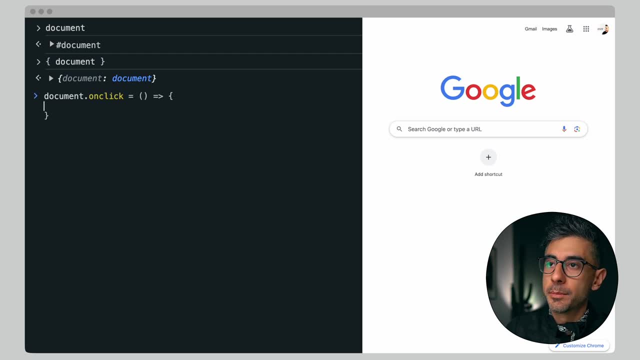 properties and methods. let's mess around with that. on click we saw. that's the first thing i want to show you. uh, let's do an arrow function function and i'm going to say consolelog: hello, dom. okay. so what do we think is going to happen? i'm going to go over here. 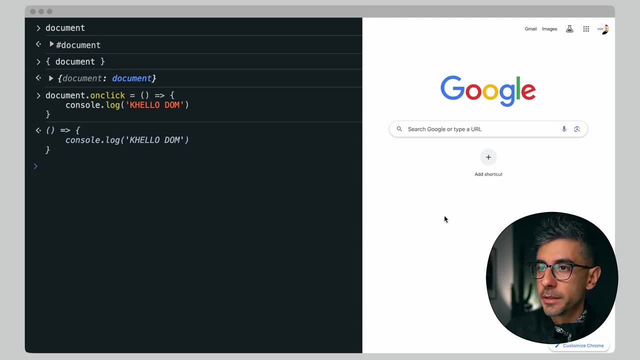 if document is truly everything, i'm going to click and i have these hidden. there we go, so i'm going to click. anywhere i click, it's going to give me this console log. now, most of the time i don't want to change the entire document. right that we don't want a, a global click everywhere. 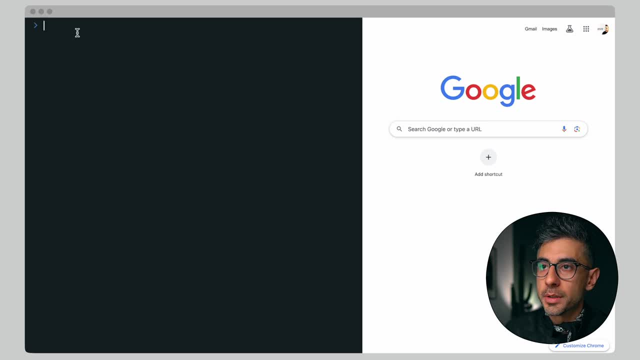 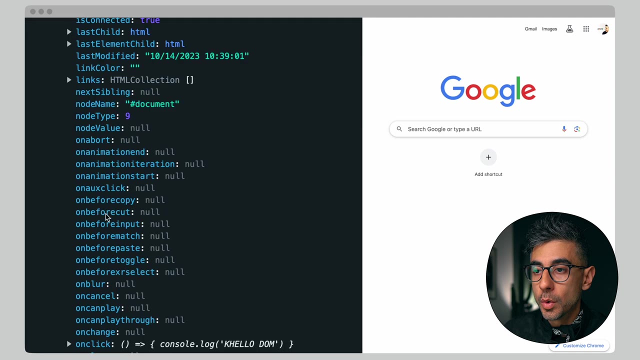 so, uh, let me get rid of all this. let's drill down a little bit into this document of ours. i'm going to go back to what i had before: document okay. so two things i want to show you here: document dot head- okay, that's uh, that's cool. and then there's document dot. 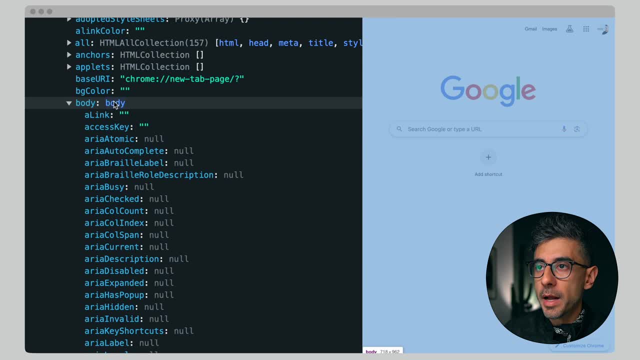 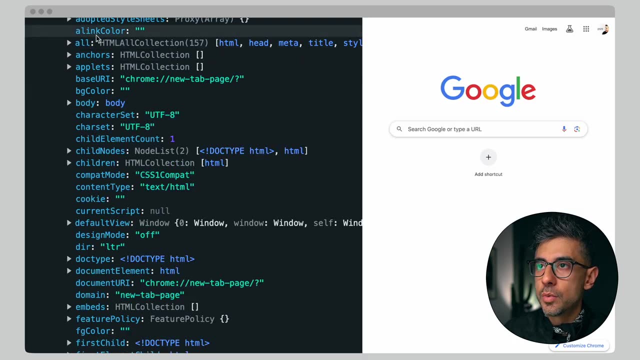 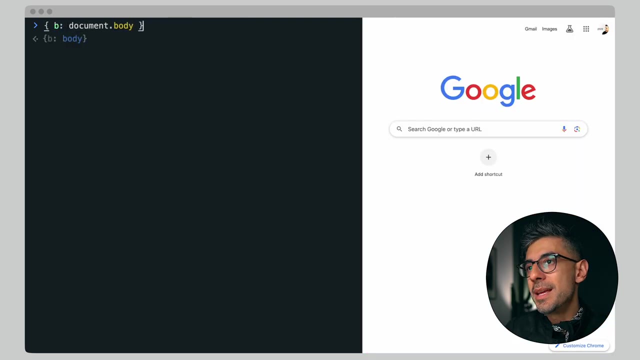 body, which is the one we're gonna mess around with. all right. so if i open body and hover over it, same thing happens: the entire body of the document gets highlighted. so let's do that document dot body. this way i can't do a shorthand, so i'm just going to say b, then we. 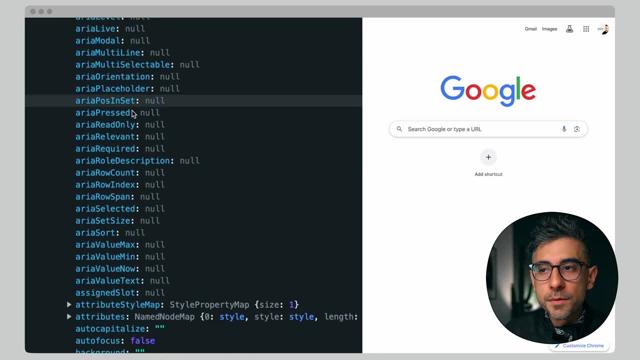 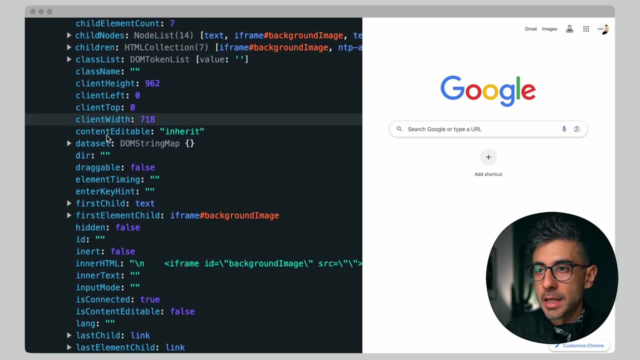 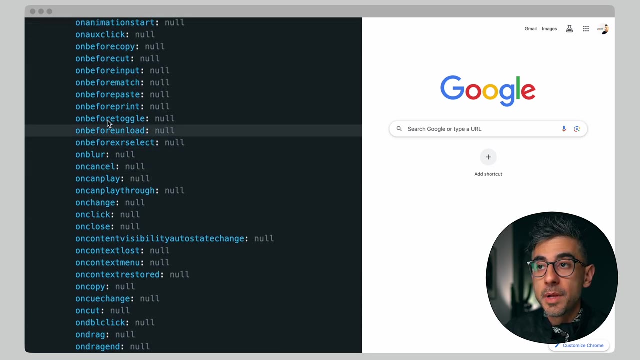 can go into b and look inside and it looks very similar, doesn't it? it just doesn't have its own body or head, but it has children, child nodes. it has the same um offsets. this is some of the positioning stuff, the, but it has all the same methods. right, we have on blur, on click. 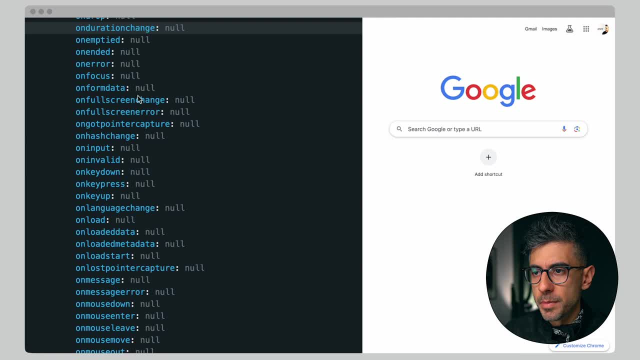 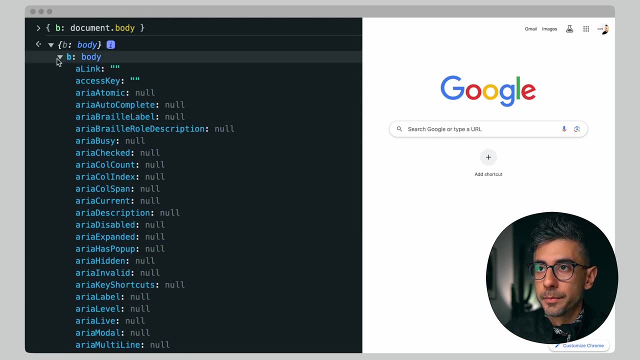 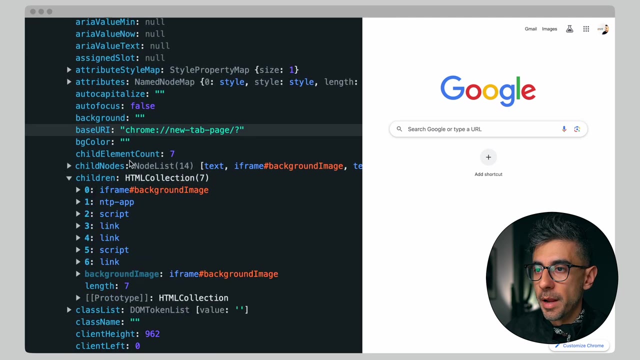 by the way, on load is might be one that some of you have used before. it's just another method. so there you go, all of it is here. let me close this. actually. let's see what's inside: body dot children. okay, there's an iframe NTP app. I'm not sure. 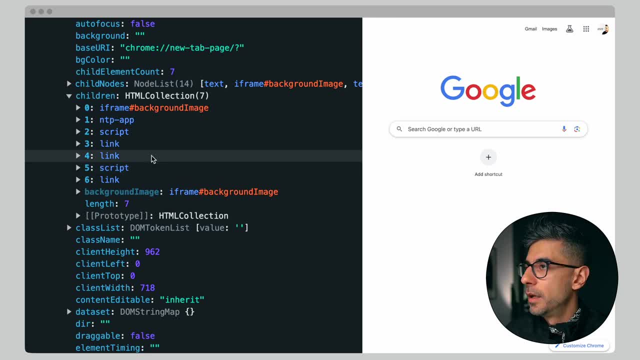 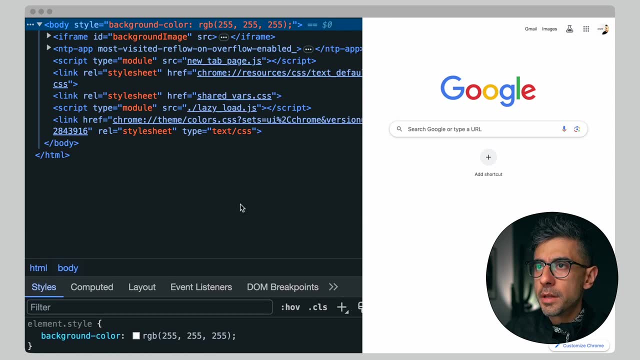 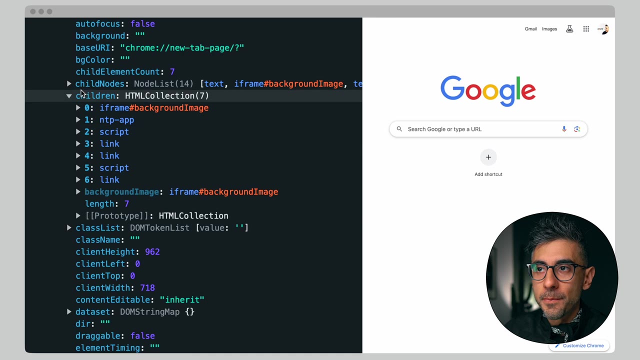 what that is: script link, link, script link. okay, so there's seven children here. let me go back to the elements. look and look at that inside body we have iframe NTP app script link, link, script link. so it seems to be that this is a data representation of exactly the child nodes that are directly under body all. 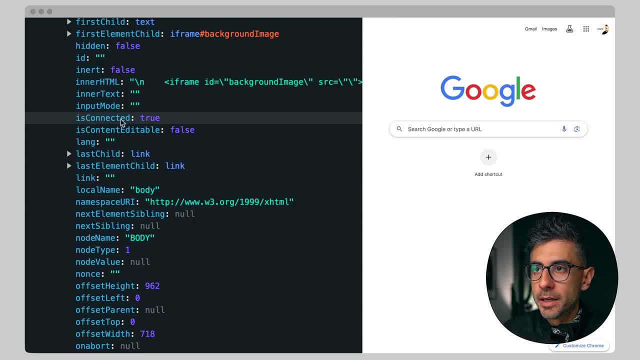 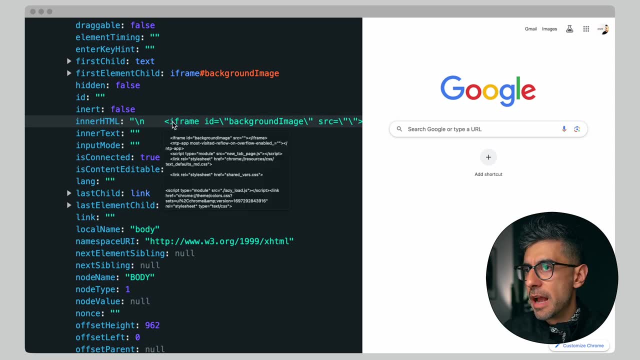 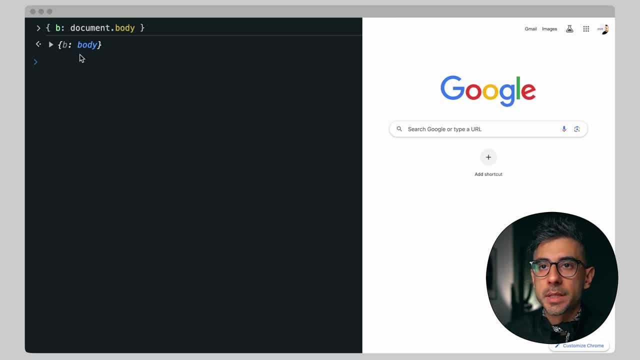 close this body again, okay. so what's the point of accessing all these elements? well, if you can access them, that means you can probably change them. let's add stuff first. I'll say document, dot, body, dot, append, so append. there's two of them: there's append and append child. what's the difference? let's try append first. 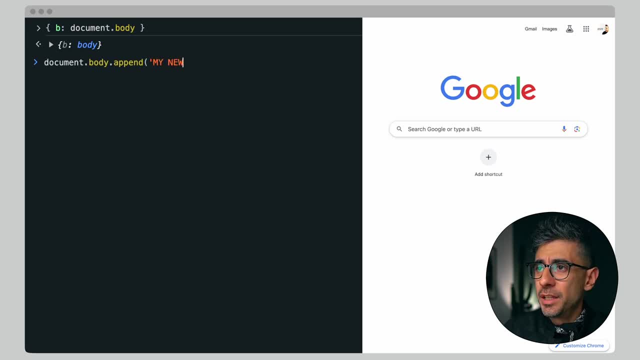 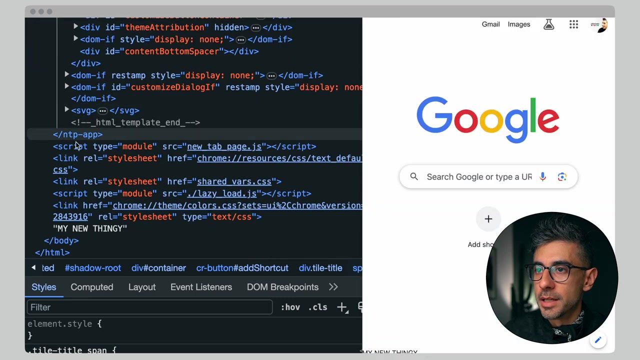 mynew thingy. Well, that didn't show up, Or did it? If I scroll down, I need to zoom in a little bit. nope, not on that. on this, My new thingy got added to the DOM And if I go into my elements I can see all the way down. there is my new thingy. 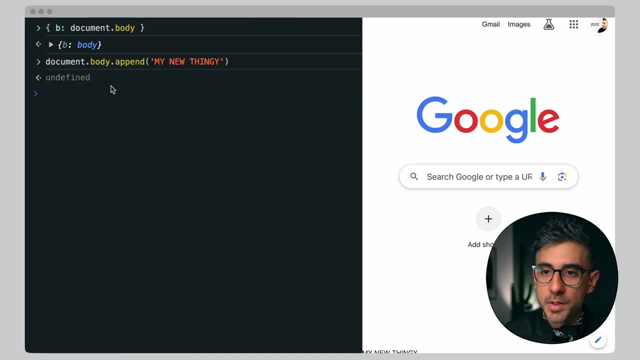 So that's what append bodyappend did for us. Let's try: append child, append child. yet another thingy: thinny ooh failed to execute. I'm going to pretend I didn't know that was going to happen. 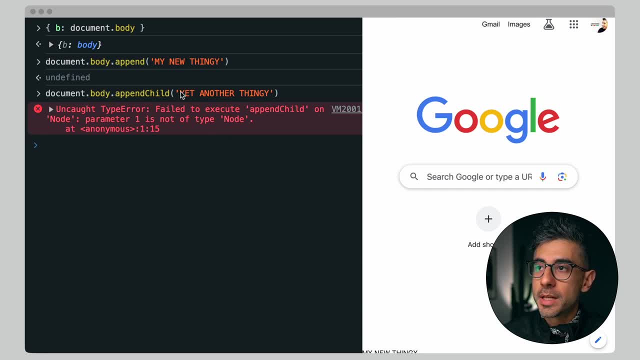 Append child on node parameter one is not of type node, So what it's saying is that you can't send me a string and assume that's going to be an HTML node. If you do append, this is going to be a text node. 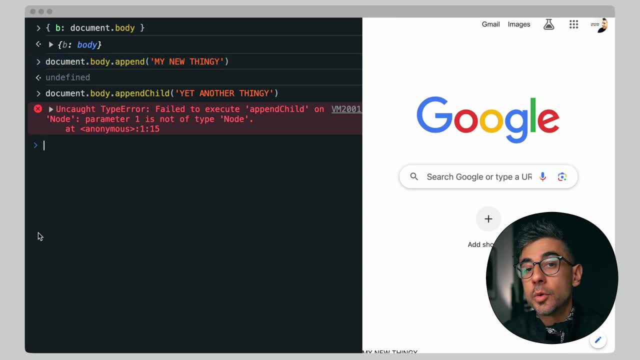 So string is fine, But it's asking for a node, So we need to create an element. If you want to add an element to the body, it needs to actually be an element. So how do we create an element? We can say documentcreate. 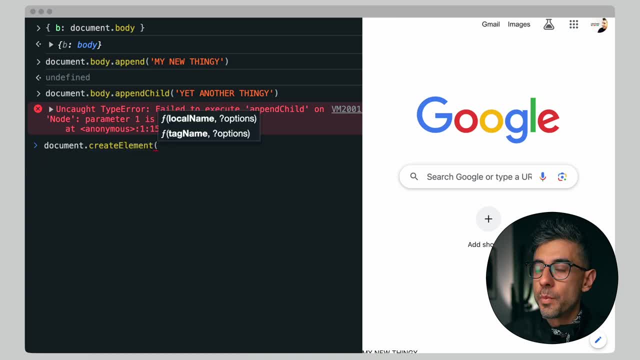 Look at how many creates there are: Create element. Now this function, this method, is telling me it needs a tag name or local name. So the tag name I'm going to use is h1.. We all know what an h1 is. 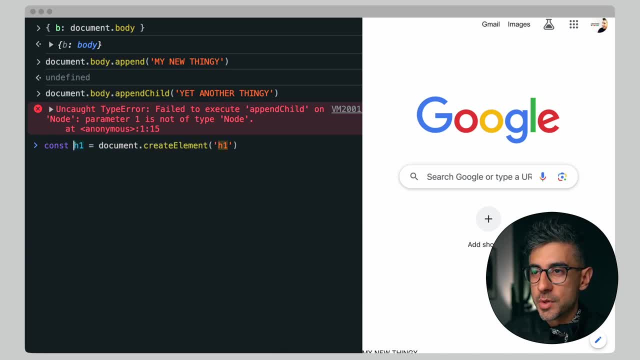 Actually, before I do that, I need to hold it inside a variable So I can play around with it. This h1 doesn't have to be the same as this h1. So just so you know my heading cool And then I can say documentappendchild, like we're doing before. 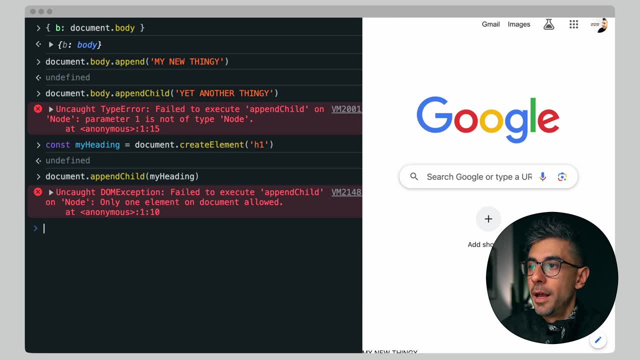 And then I'm going to add my heading. It doesn't work again because I added it to the document. I need to add it to the body. Okay, it returns the element itself, h1.. I don't see it here. 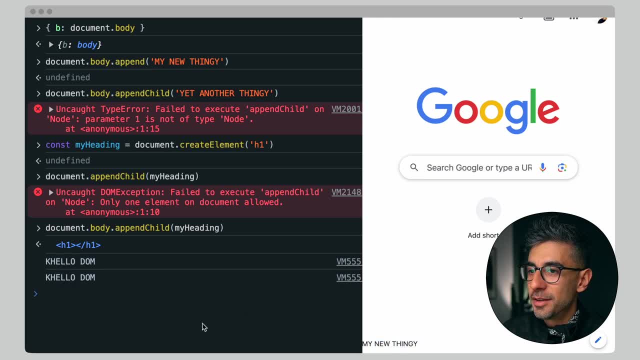 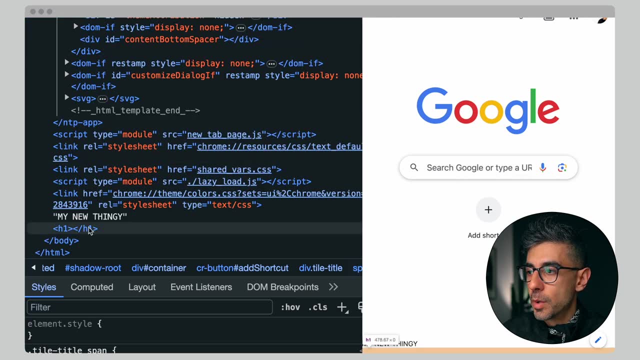 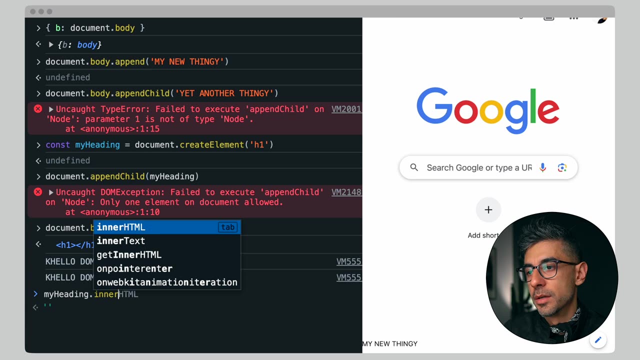 Well, Let's go down. There's a little bit of gap here. That's not good, But if I go into my HTML you can see the h1 is there. But the good thing is I can say myheadinginnertext. let's say equals. I am your header. 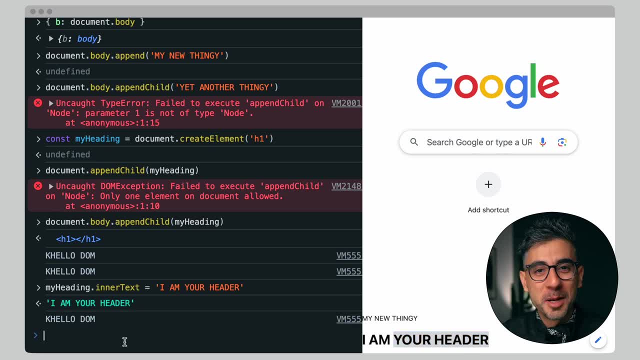 And it showed up here. Booyakasha, Look at this. I'm manipulating the DOM, adding things. This is cool. I'm going to change it now, That's. what's nice about this is that these are just JavaScript objects. 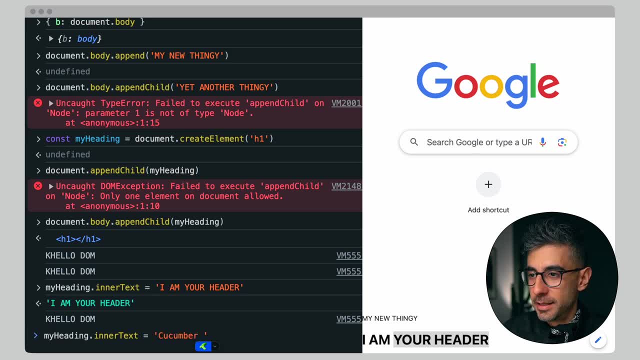 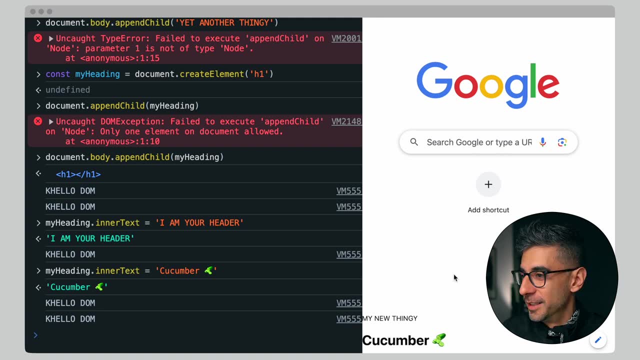 I'm going to say kukumba And let's see if our- Oh, there we go. Thank you, macOS. Kukumba Makes your bones stronger. Let's do something else Instead of adding something useless like kukumba. cucumbers are not useless. 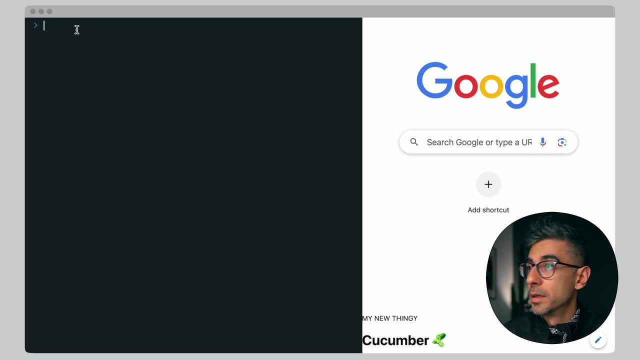 How about we try to add the current time? Yeah, Current time. I'm going to do something really not great, because I told you we shouldn't be doing this in the beginning. Can I change the inner text? Okay, So I just killed the entirety of the body. 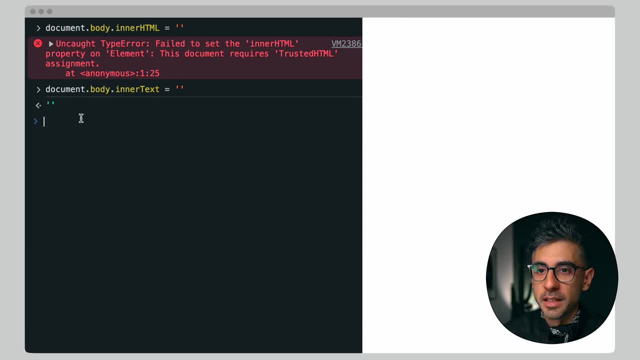 So please don't do this, But I'm doing it so we can get rid of everything and I can show you a little easier. So I'm going to refresh, actually, and kill the HTML one more time. Okay, Everything is gone. 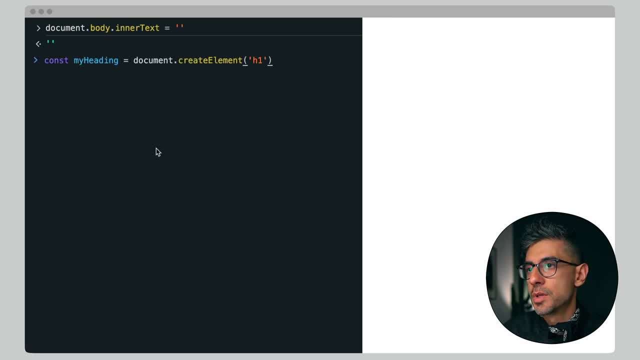 Everything is awesome. I'm going to copy pasta from my notes. So my heading: I'm going to create a heading, Then I'm going to add it to my HTML. I know it's there because we saw that, Just to be clear. I'm going to do this in the meantime, that inner. 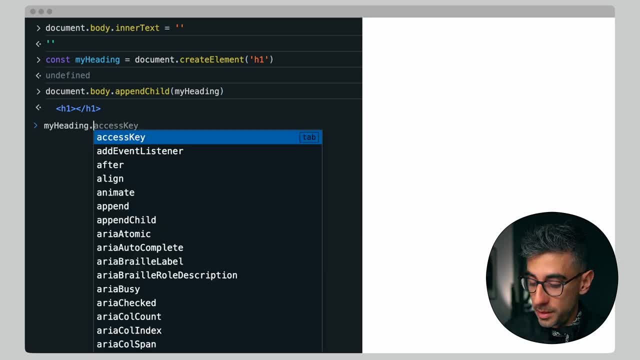 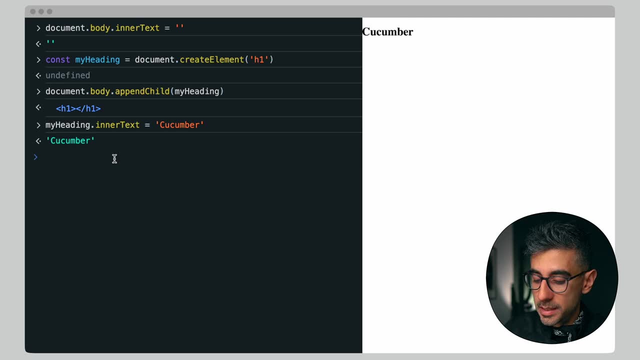 I can even do this to prove that it's there. Chrome tries to be too smart. Inner text equals Cucumba, So that's there, Okay. So now, what I'm going to do is const now equals new date. I don't know if you're familiar with the date function. 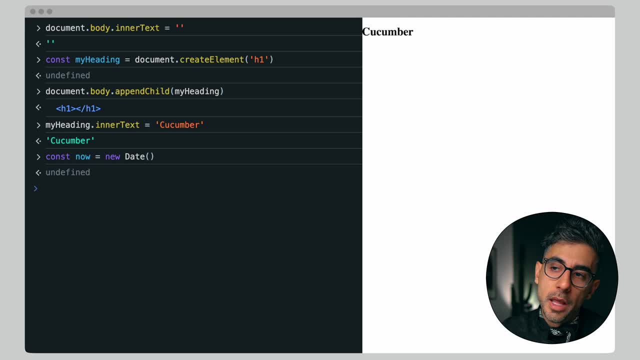 If you're not go to MDN and check it out. It's pretty cute. And then I can say my heading dot. inner text equals Let's do a little string literal And I can do now dot. So now is an object that represents the. 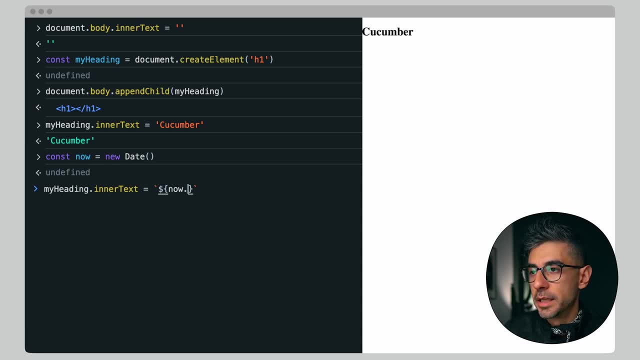 It represents the current date and the current moment. I can say: now dot get hours, So what is that Ten? It's ten in the morning And I can put one of these in there and do another. I don't need. 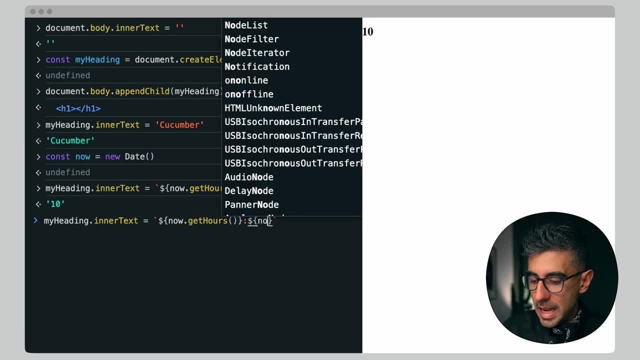 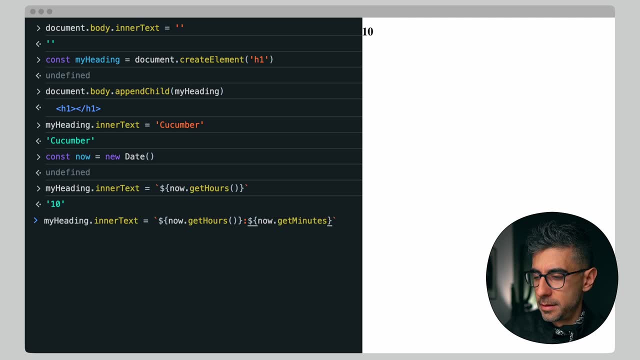 I need this And do now dot get minutes, Minutti, Minutes, Minutti, Minutti. What time is it? 1048.. So that's useful, right. That's probably how you can go about updating the. 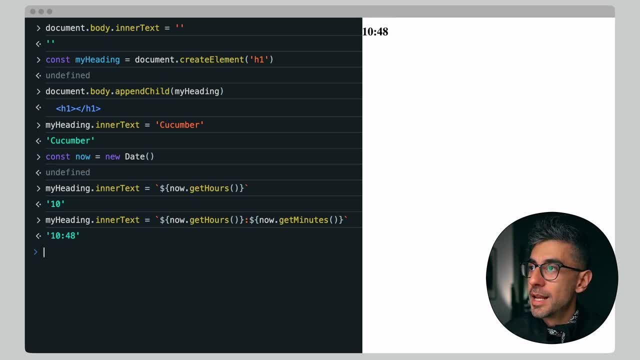 time on the page. If you've been to a website where it says what time it is, it's actually grabbing the time from my machine, from my locally set time, which for me is just to what the internet says. it is because I trust the internet. This should prove that we can actually grab dynamic. 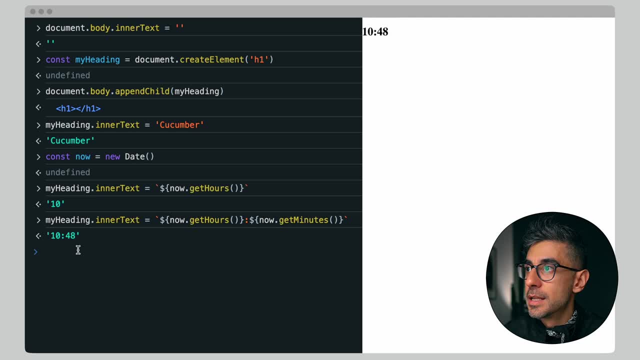 information and drop them on the DOM. It doesn't have to be static content, So we just turned this into a mini app that shows you what the time is. So if you run this exact same code on your machine at a different time, or even on my machine at a different time, it's going to result on something. 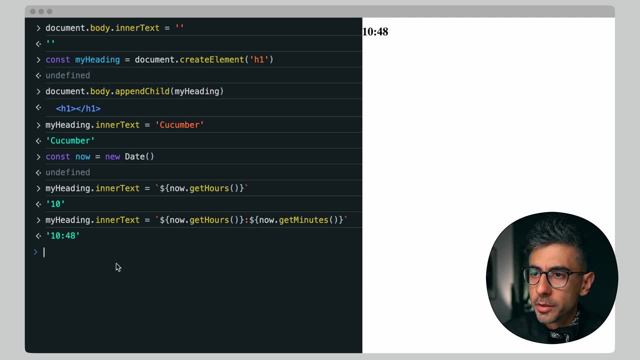 different on the DOM, which is very, very cool. A quick note here that this time isn't going to update because this code only runs once. It runs only the one time that I execute it. You can set an interval or a timer, or set intervals is probably. 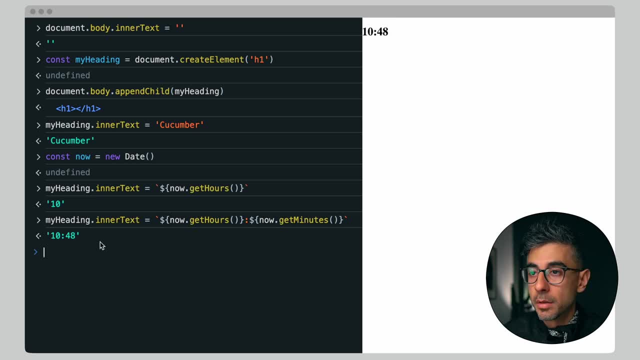 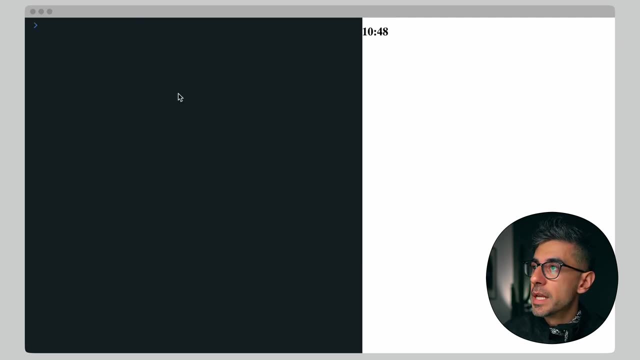 the way to do it, where this can repeat once a minute or whatever, but just know that this time isn't going to update automatically. All right, I'm going to get rid of all this, And what we're going to do is now build a useless to-do app. To-do apps are pretty useless, but that's what. 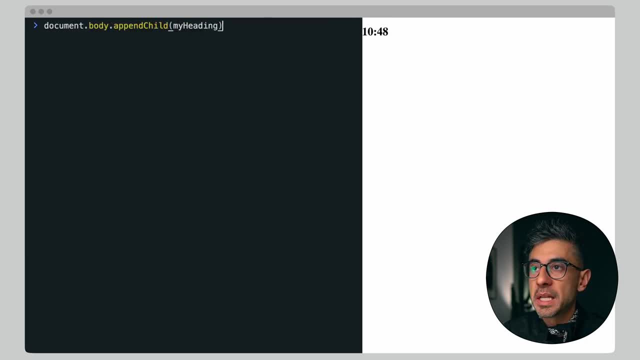 we're going to do, because it's going to show us a lot of interesting things that we can do with removing and event listeners And a few other things. So I'm going to do the terrible thing again and get rid of everything in the DOM. So now I'm going to create const input. So what is a to-do app? Let me zoom out for a. 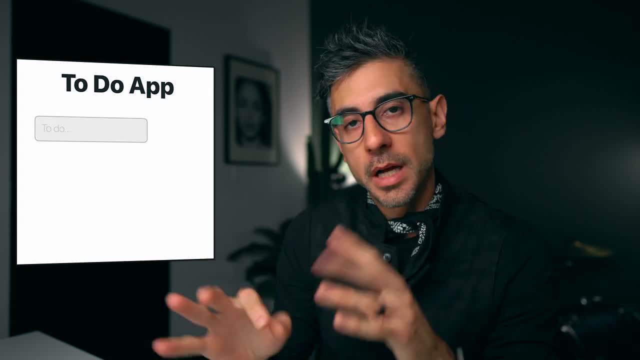 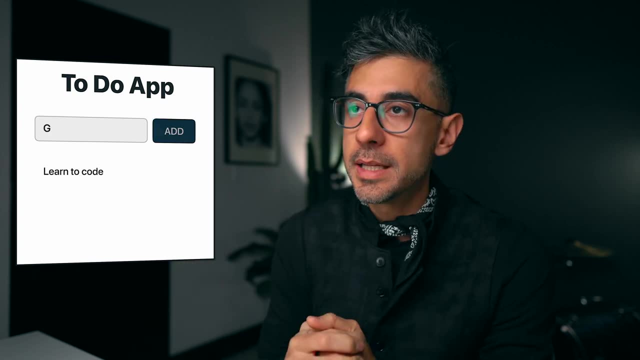 second, A to-do app has an input where you can type the thing that you have to do. Then it probably has a button where you can submit that to-do to be added to your to-do list. Then there's, of course, the list itself- all the things that you have to do. 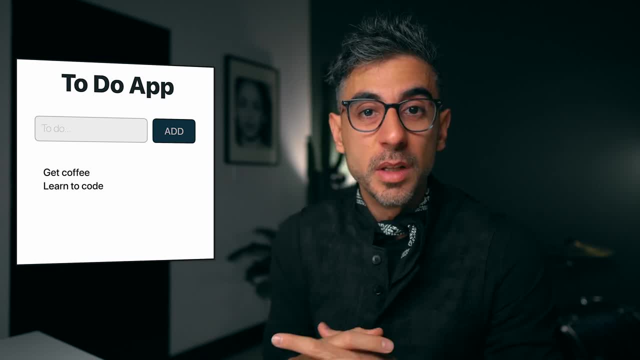 And you should probably have a list of all the things that you have to do. And you should probably have a list of all the things that you have to do And you should probably be able to remove things from the to-do list right, There's usually a button where you can. 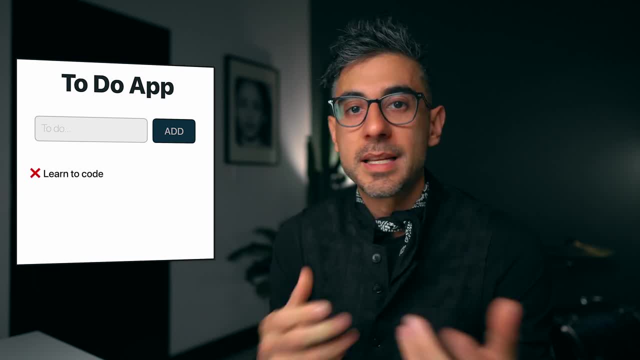 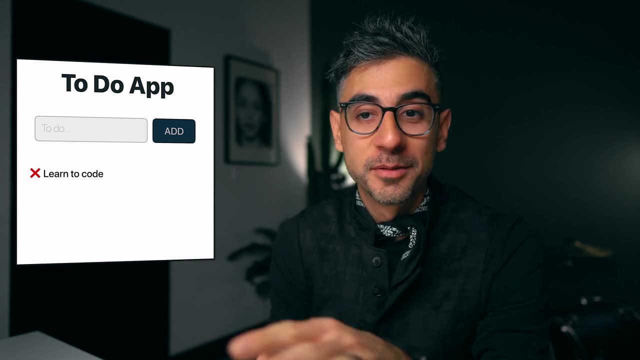 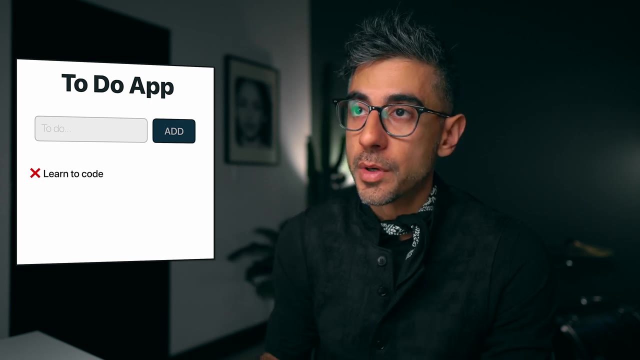 click it and it removes the thing and it says it's done now. So we're going to try and create this with- I'm going to hope for- about 10 lines of code. I haven't counted how many, but I'll show you how easy it is to build something like this in the DOM using just JavaScript. 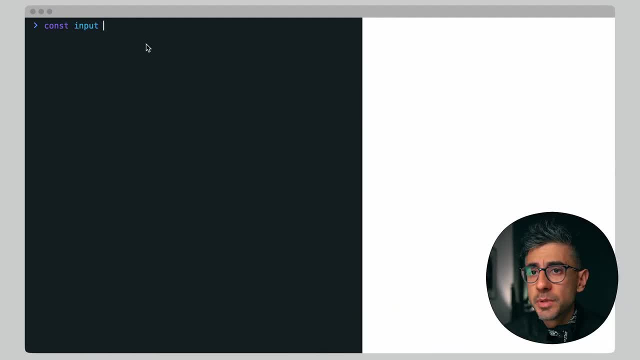 Okay, Back to the browser Browser. I've missed you guys. So let's create an input Document. just like before, just like the heading, I'm going to create document that creates elements, create element there. What kind of element do we want? We want an input. 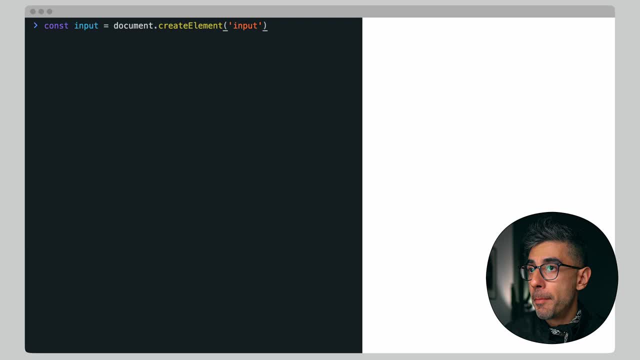 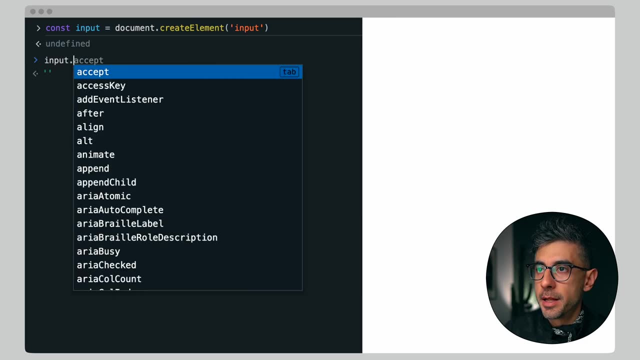 Don't just put input here. It takes a string, but it has to match the type of the tag name that you want. All right, I have an input. Should we add it to the DOM? Well, let's play with it first. 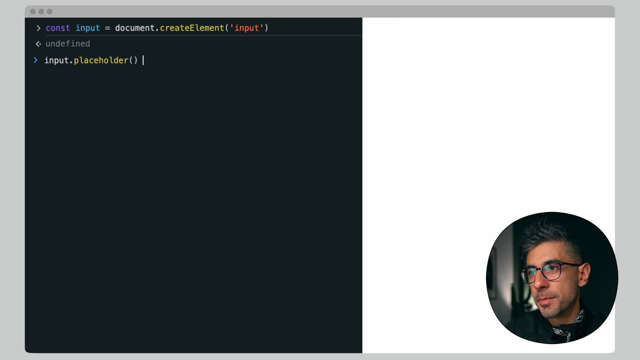 Input has a thing called placeholder. It's the little text that shows up there Inside the input. I'm going to say add: doodoo, Fine, I'm not feeling particularly creative today, Do you feel it? I feel it. Documentsbodyappend- child Input- Input. Look at that. All right, It doesn't look great. 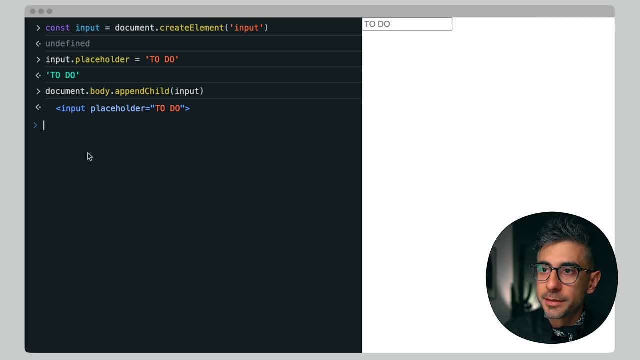 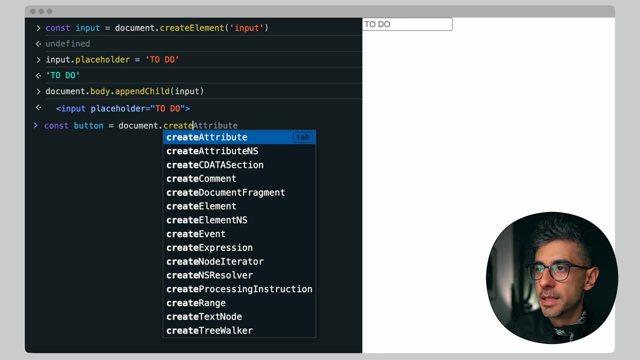 I'm going to zoom in a bit. It doesn't look great, but it's there, Cool. Next thing, Let's add our submit button. equals same thing: DocumentscreateElement. And as you start doing this stuff, you start to notice why some of these frameworks have come into play, because 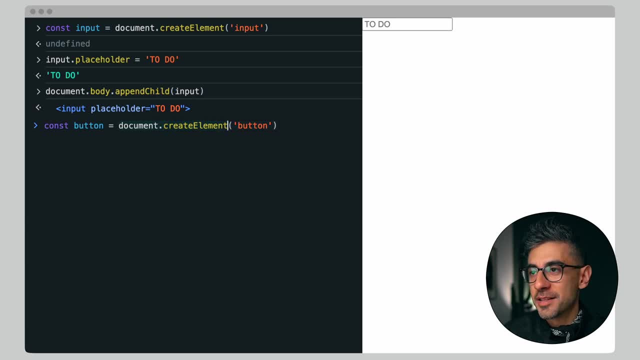 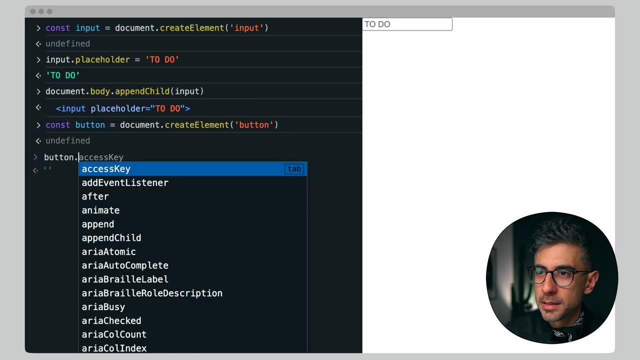 the DOM API is a little bit redundant. It kind of sucks to always have to create elements like this. but now you know, All right, Let's do the button, The button dot. How do we do the label? I think it's just value equals add. let's just call it add. all right, let's hope for the. 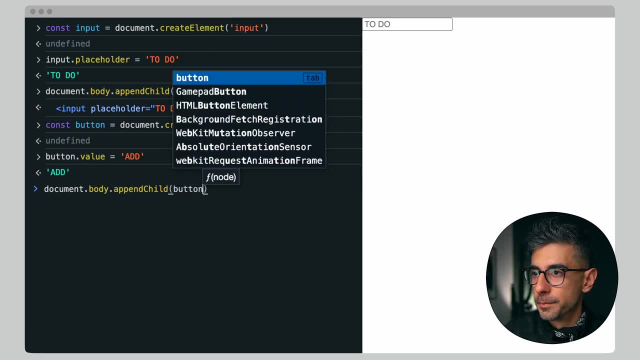 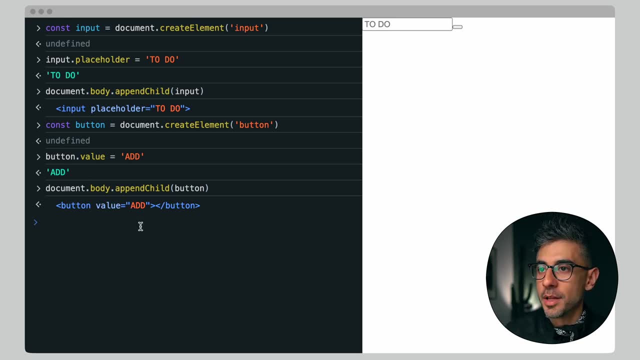 best and then up we're gonna append it button. oh, it wasn't value, it's what is it? I have notes here. I can well inner text- that's the note I wrote, which is not great, but whatever inner text add. cool, all right, we have a button it. 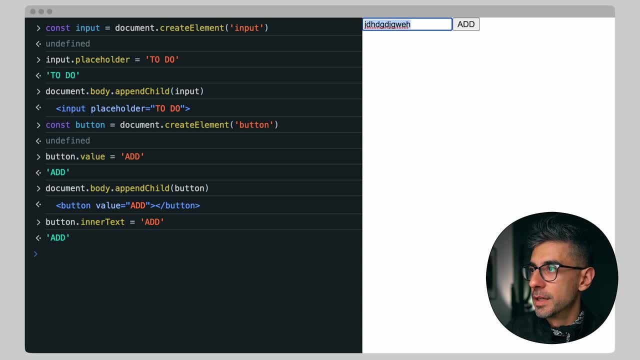 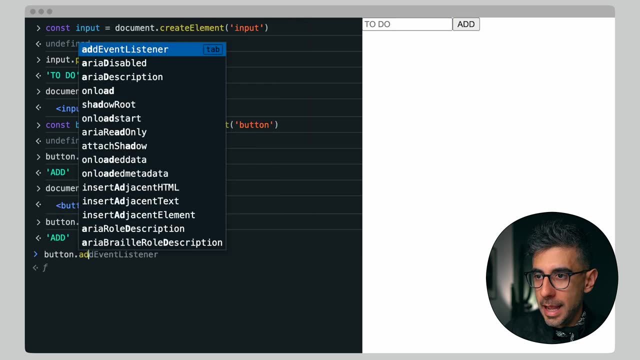 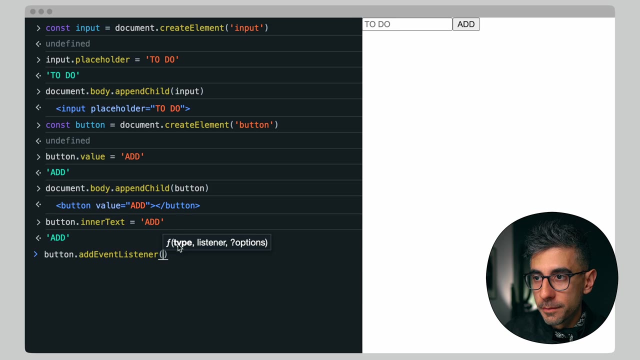 doesn't do anything right and the input, it doesn't do anything. so let's add a event listener to the button button dots. add events listener. we can say so, look at this, the type of the event, and then the listener, the handler itself, and then we have some options which is optional. so the type is on, click on Calick and 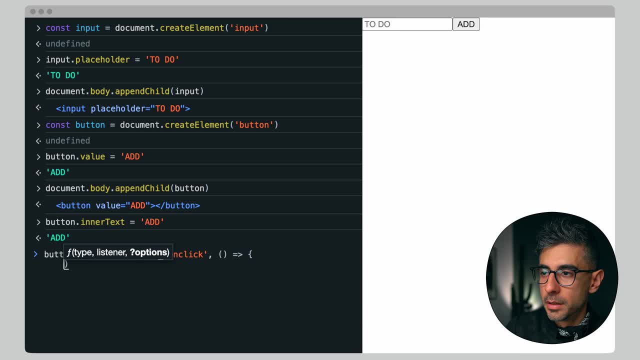 the list has to be a function. It can be a reference to a function or we can just write it here online. So I'm gonna say, to start with consolelog: You clicked me, dude, Is that everything? Okay, let's see. 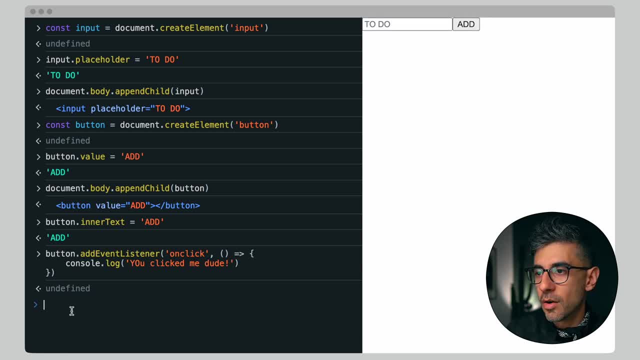 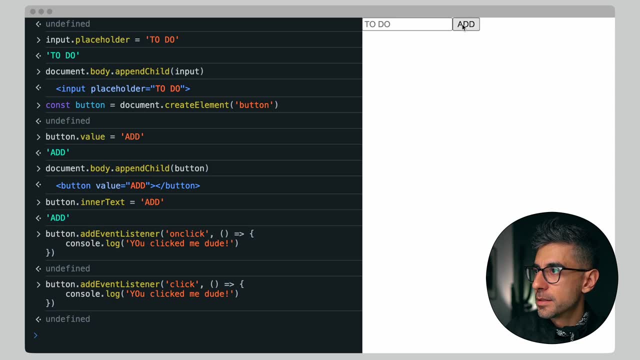 Add. No, it doesn't do it because it's not on click, it's click. What are you doing? All right, let's see. Okay, you clicked me, dude. I have a typo here. Terrible at that. 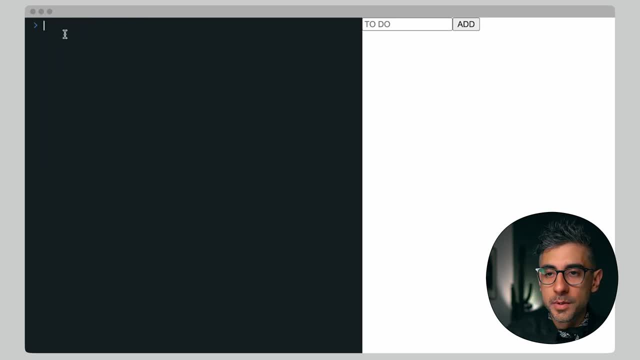 I'll get rid of all this so we can go back to the top. So this way you can see a little easier. Instead, I wanna add a click where: what does it do? It grabbed the value from inside the to-do. learn to code. 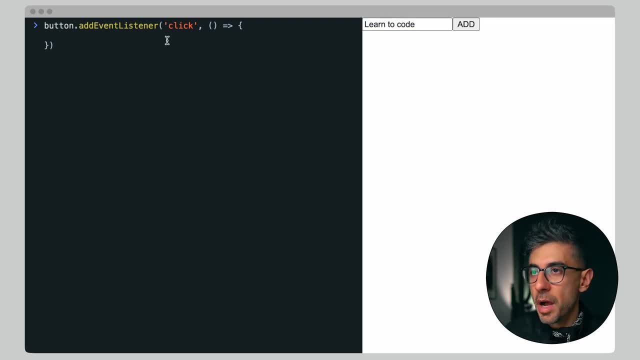 And it does something to it. Maybe it creates a div and adds it to the body. Yeah, let's do that. What is inputvalue? So const equal? actually, let's create our div First. equals documentcreateElement div, And we've been naming these the same as the type of tag. 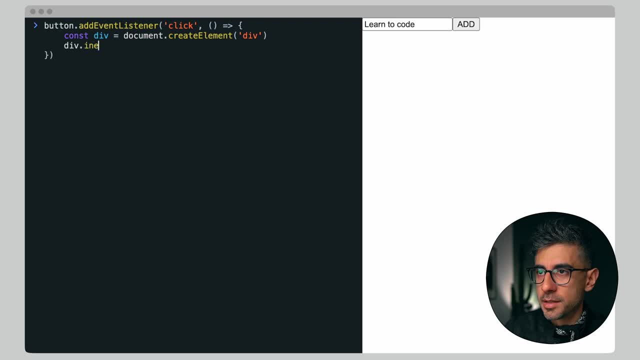 but they don't have to be. as I mentioned, Divinnertext equals. I'm gonna get some shit for using inner text. Just cool it guys. Just use whatever is better. Actually, inner text is not so bad. It is supported in pretty much every browser now. 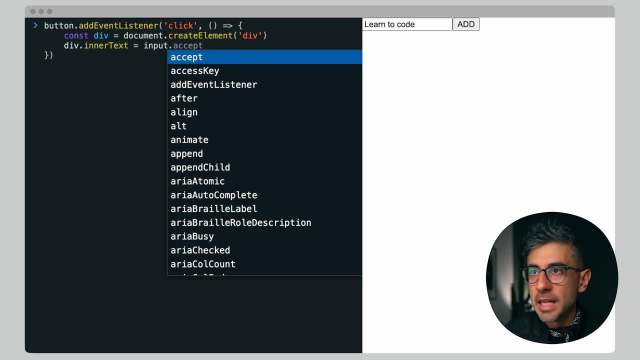 So if you wanna be particular about using a method like there is a setText or setHTML or something like that, there are other ways to do it, But the point here is that we're doing this dynamically: Inputvalue. we do that. 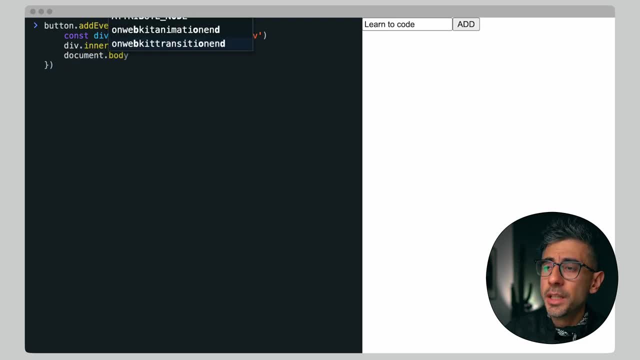 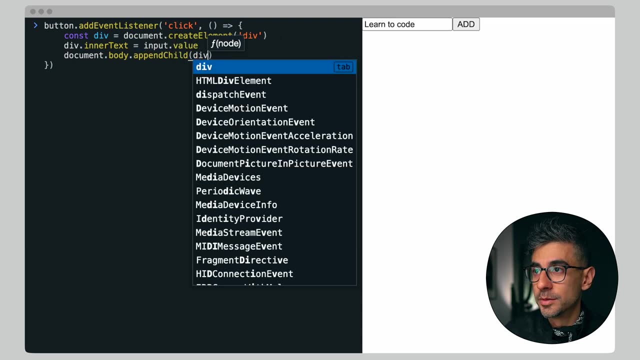 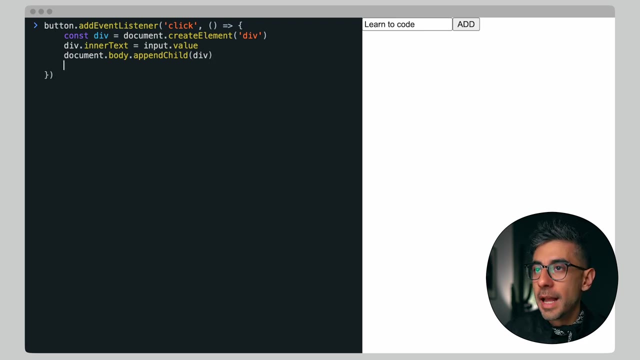 And then documentbodyappendChild. It's starting to get repetitive a little bit, isn't it? So you're starting to- yeah, You're starting to appreciate- React a little bit. Okay. so let me see, did I change anything? Okay, and then what I had was: I'm gonna grab. 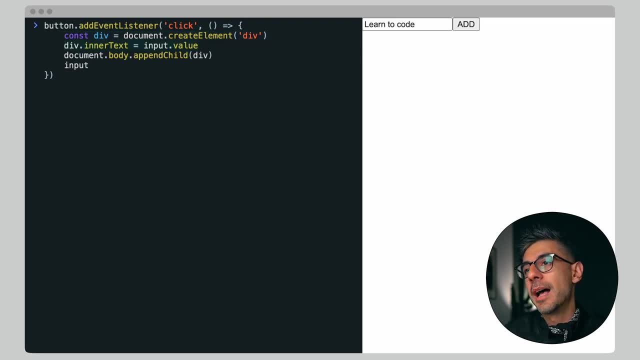 so I'm gonna create a div element, I'm gonna add the value of the input at that point when the thing is clicked into the div, And then I'm gonna add the div to the document And then I wanna get rid of, I wanna get everything out of the input. So I'm gonna clear the input. So I'm gonna get rid of everything out of the input. So I'm gonna clear the input. So I'm gonna get rid of everything out of the input. So I'm gonna clear the input. basically. 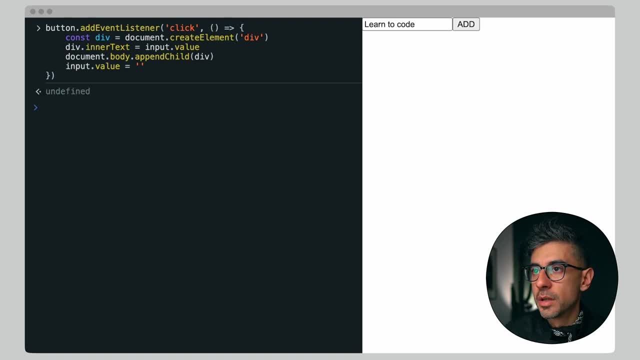 Okay, should we do this? Let me see. let me check my notes. Everything looks good. All right, let's see. So learn to code. It worked, All right. let's take a look at the elements. Body: we have an input. 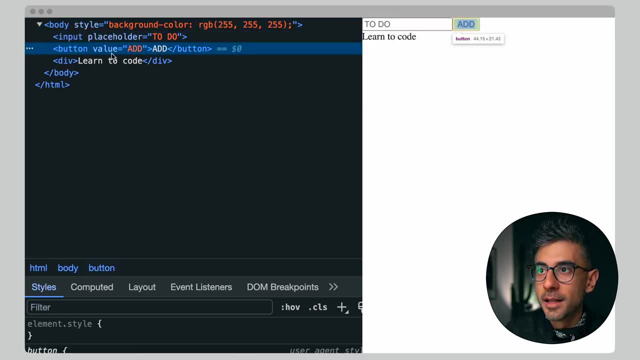 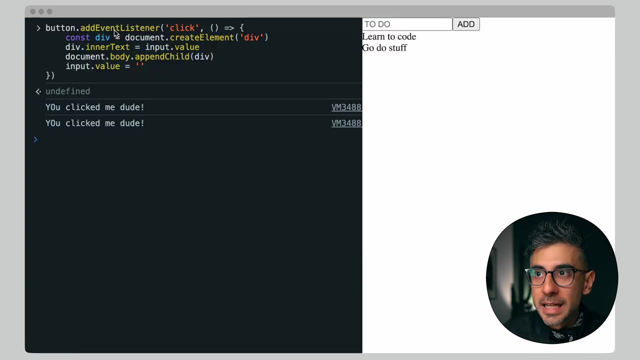 We have the button that has a text inside add, And it said: learn to code, Let me add some more. Go do stuff. It gets added. So every time we click this thing, this entire function runs, which is very, very cool. 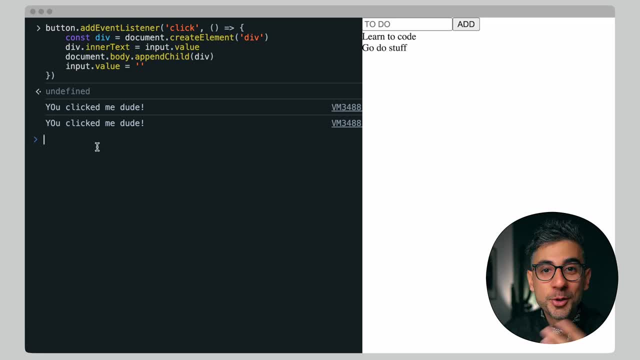 So you're manipulating the DOM here, dude Or dudette, We're adding things and we're removing things. We're not removing things yet. We have event listeners, But we can remove it, though We can say: when I click on each of these, you can delete it. 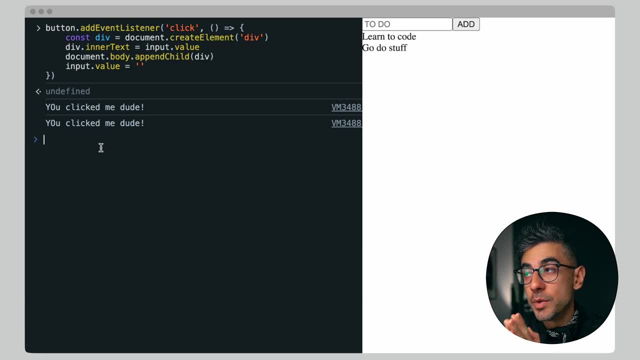 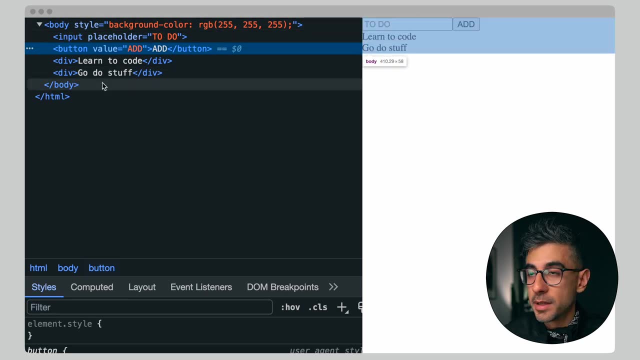 Before I do anything else, I wanna make sure we do this using something else. I'm using semantic HTML. This is terrible. What I have here is what amateurs do? They just drop things on the DOM. They don't care about semantics of HTML. divs, divsoup. 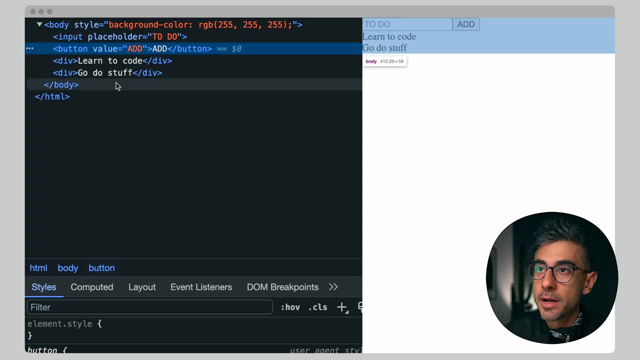 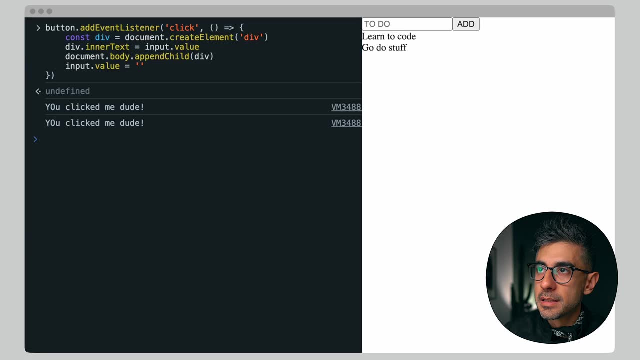 We don't want a divsoup here where you have, like, lots of different divs and different layers. If you have a form, like I do, an input and a button, it should be inside a form so that some browser default things like pressing enter 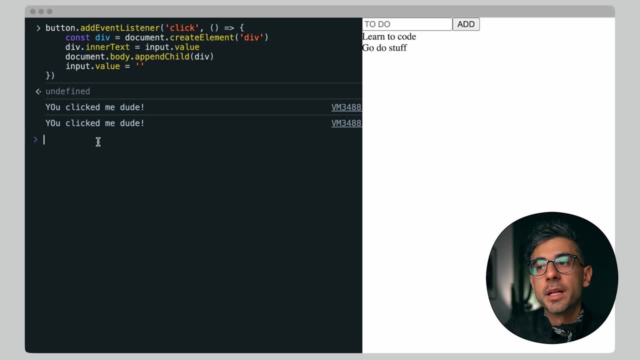 and stuff like that by default works. So we're gonna take this, We're gonna take this, We're gonna take this and convert it into semantic HTML. So I'm gonna copy paste some of this so you don't have to watch me type it again. 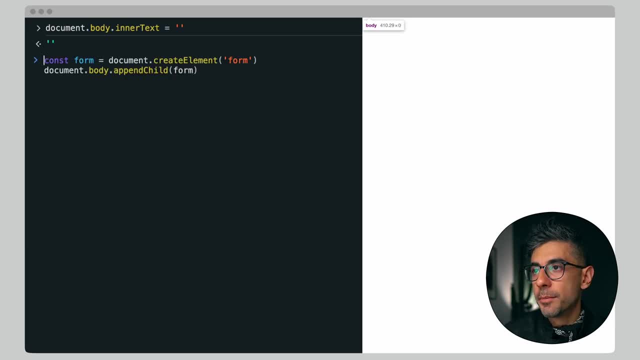 Let's get rid of everything in the document, in the body. I'm gonna create a form element, So let's type form. I'm gonna append the form to the body. Then I'm gonna do the same things. I'm gonna create the input and add to do. 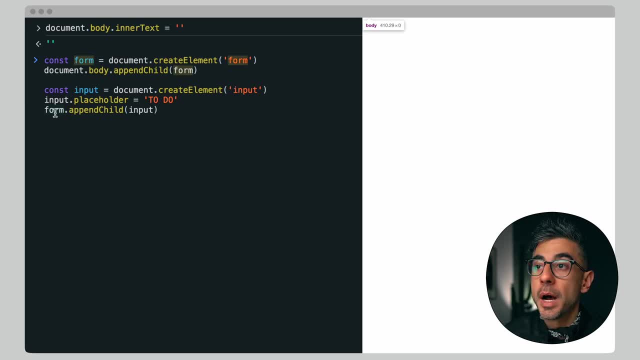 but then I'm gonna say formappendchild instead of body: documentbodyappendchild. So I'm gonna add the input to the form. Then I'm gonna do the exact same thing to the button. I'm gonna add the, let's say, add submit. 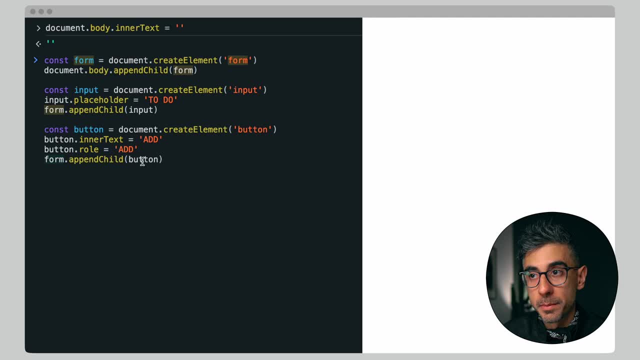 What is this seriousness? submit. So then formappendchildbody. So I have a form that got added to the body, and then I have an input and a button that get added to the form, And then, instead of just adding the divs to nowhere, 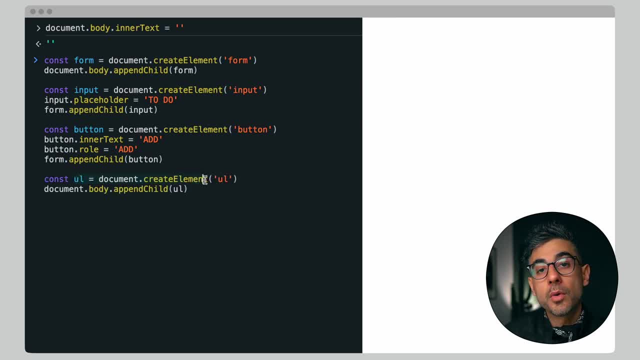 or to the root of the body. I'm gonna create an unordered list, a URL and the URL I'm gonna add to the body And then, on form, submit this. I probably should write: Form has a on submit And the reason why it doesn't auto-complete. 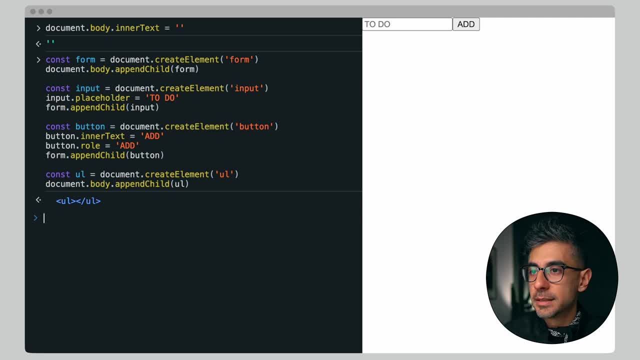 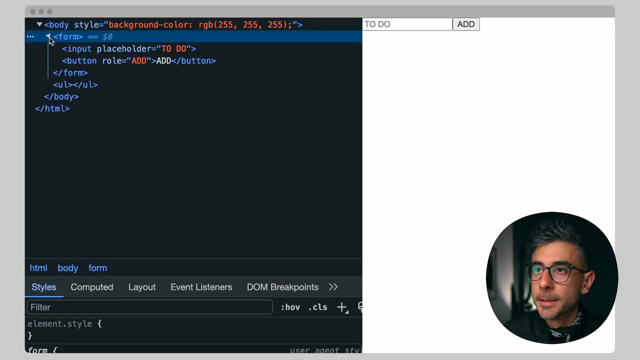 is because it doesn't exist yet, So I'm gonna press enter So everything gets added. This is fantastic. So if you want to see it, Sure, I'll show it to you. Craig, we have a form, So now you can see, you can add things to. 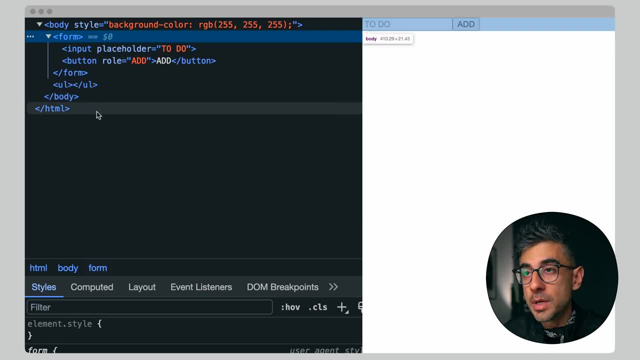 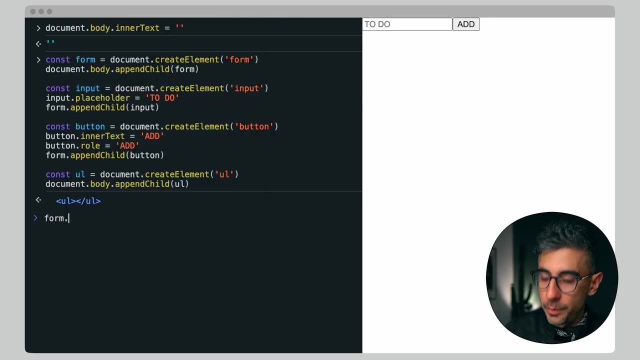 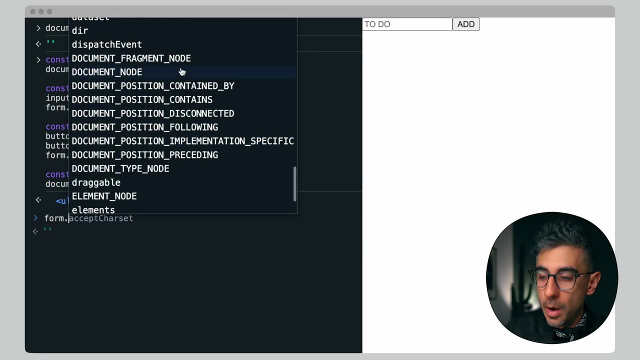 not just to the body but to any other elements. If you have a reference to it, like I do like with the form, I can add things to the, to the form. so now I can say form dot, press dot, and all of the Attributes and all of the functions that I can do show up here on. 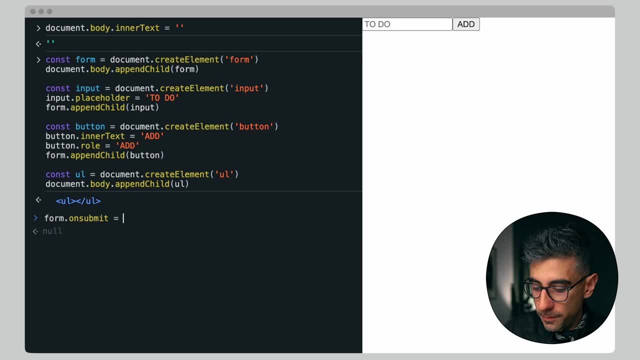 Scroll no on submit Beautiful. I Can then add a an arrow function here and say: I'll do that at the end I'm gonna create a list element and this does not have to be typed again because I've already done it for you: List element. so Li, which is a list element, semantic HtML, life here. 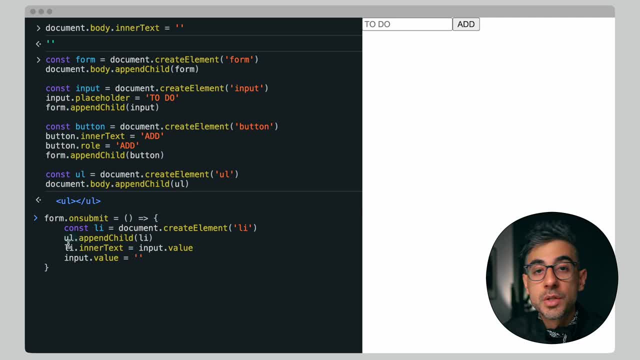 And then I'm gonna add those allies to the ul, right. so we have the form and it has a sibling. That is the unordered list. the form has input and a button and the unordered list is gonna have list items: the allies. the one thing I have to add here is e. 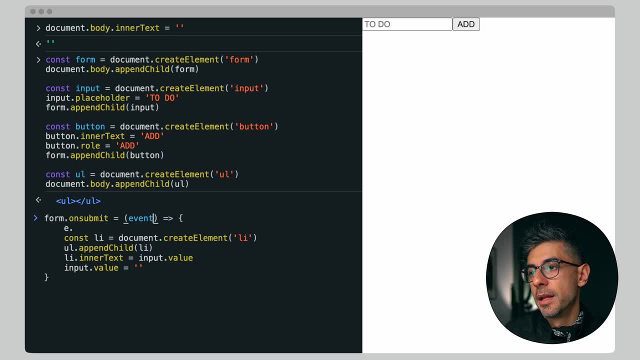 Which is coming through here, or I should say event Is a parameter that gets passed into every event. Ah no, I messed it up. There we go. I'm gonna say event dot Prevent default. the reason why I have to do this is why I have to do this is because forms by default when you submit. 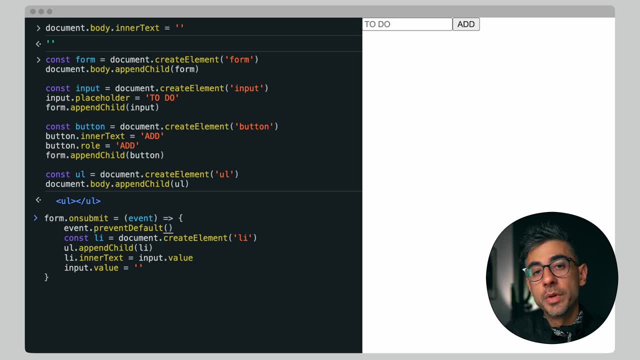 them. they Actually are supposed to redirect you somewhere else. so if I don't do prevent default, this page is going to refresh, since I don't have a URL where it's Supposed to go to. so this is a larger discussion We have to leave for later. 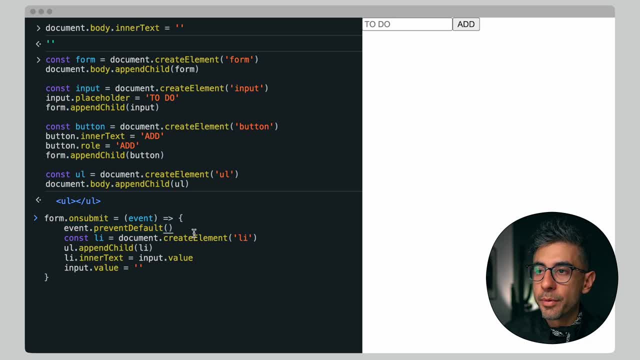 It's about how events work and propagation and why preventing default is necessary a lot of the time when you're writing JavaScript, So just take my word for it. I'm gonna come back to it in a different episode and explain why exactly. so let's add this: 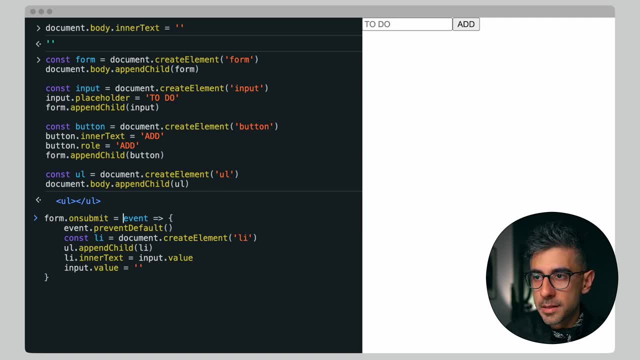 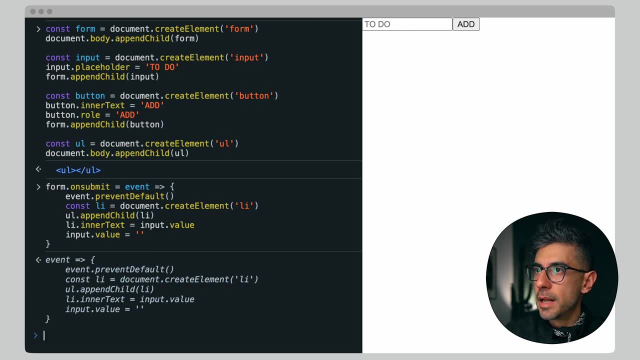 I think that's everything and, by the way, I can get rid of this since there's only one argument going into my function. Let's press enter and see what happens. Okay, let's inspect an element. Not, not much actually has changed. We have the UL. Let's add our stuff learn. 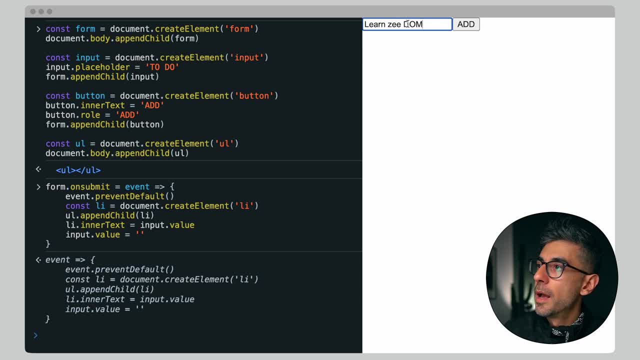 Z Dom. Okay, I'm gonna first press the button shows up. great, then I'm gonna go learn other things. This time I'm gonna press enter on my keyboard. Why did that work? because we're inside a form that has a on submit event handler. This is why you want semantic HTML. 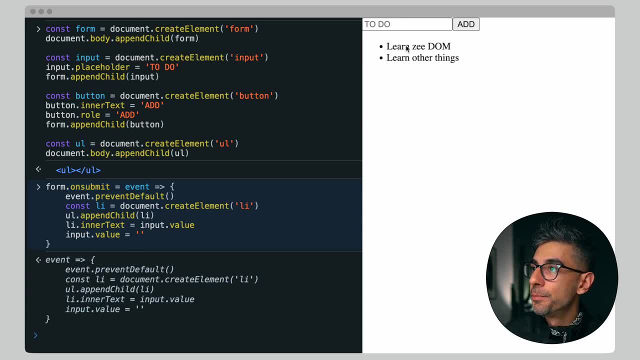 This is why you want to use the right element for the right thing, because you get this type of behavior without item right a on Key down, which is the event for capturing keyboard events. I don't have that, but so this means I can just type and type and type and. 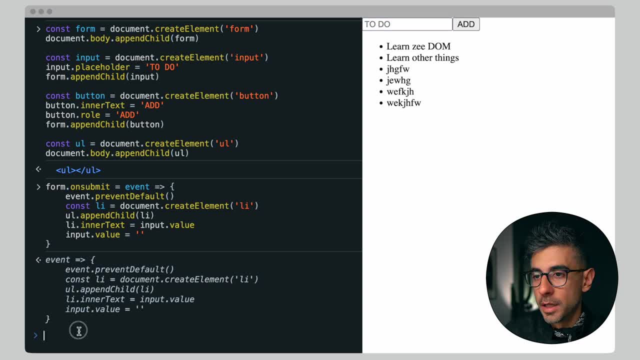 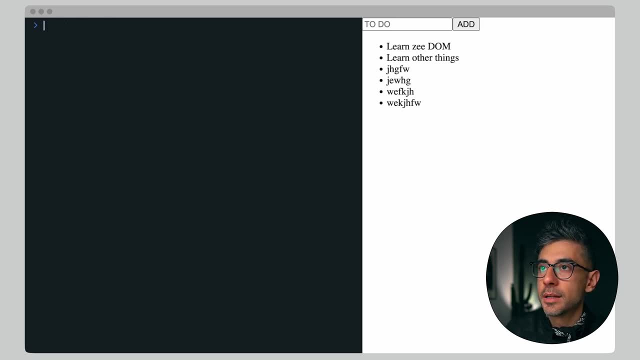 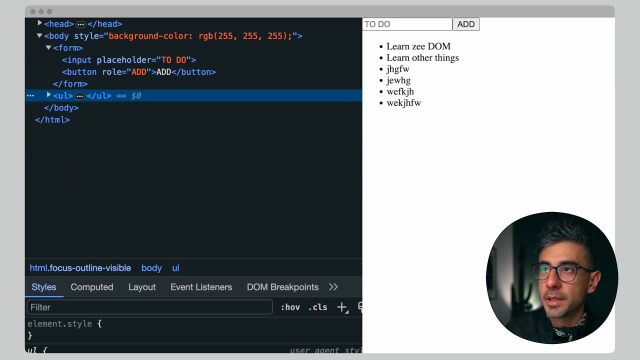 Keep going and I don't have to every time go to the button. So let's try and now add this functionality where we remove the allies. Actually, let me take a look at the elements. Li, yeah, so all the allies are here and they all get added dynamically. 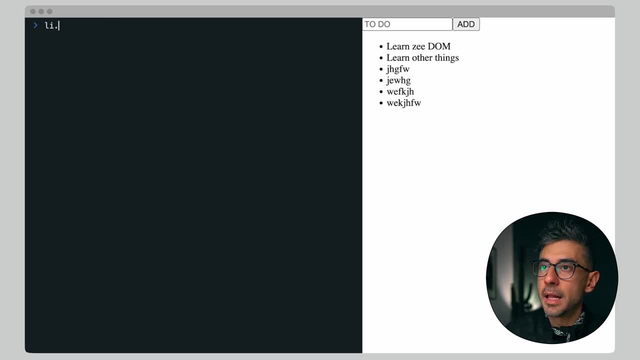 Okay. so now, if you want to remove the elements so I can say Li, dots on click. I'm not gonna add a button next to it for the purposes of this video, I can just say: Every time you click anywhere on the Li, I can say Li. 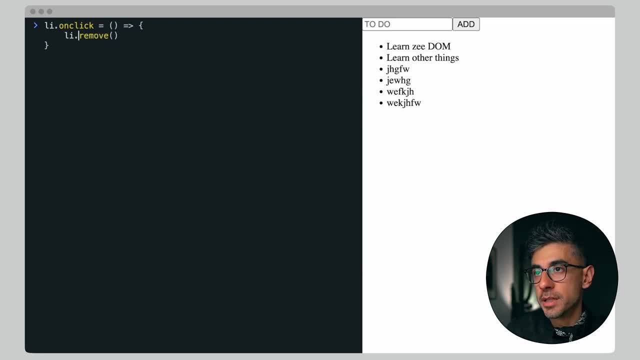 Dot remove, which is a function that every HTML node has, where it can just remove itself. So if I do that, oh, a lie is not defined. There is no reference to the Li. so What we're gonna have to do, we're gonna have to. I'm gonna have to do this again. 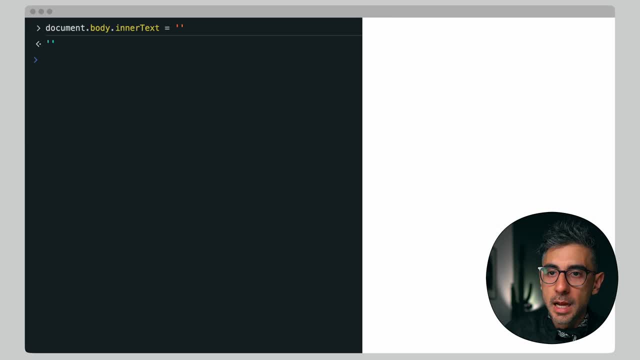 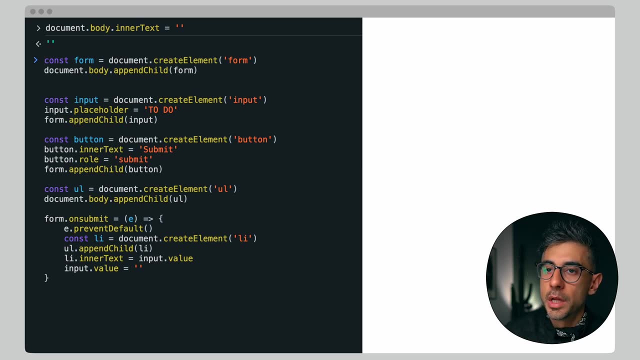 I'm gonna have to refresh the page, copy pasta, the entire thing, and obviously this is not how you develop. You develop in your IDE. I'm in the chrome dev tools Just to demonstrate. stuff where we have reference to An Li is here. it's inside this form. on submit function. 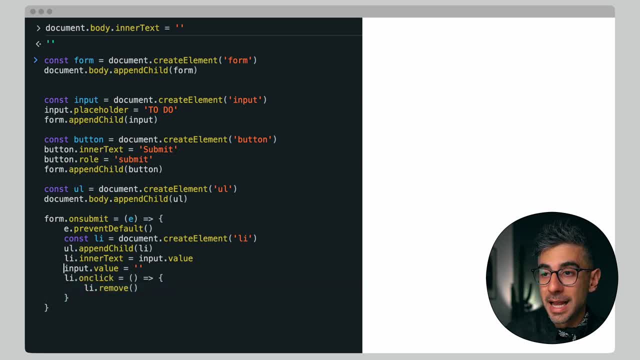 So what I can do is I can actually put it right inside here where I have access to the Li, while I'm customizing the Li, Adding inner text and stuff like that At I can add event handler, the click on click removal Functionality to the Li, so that way, every time an Li is created, 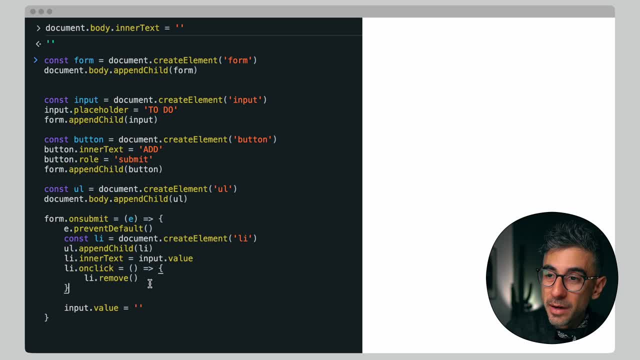 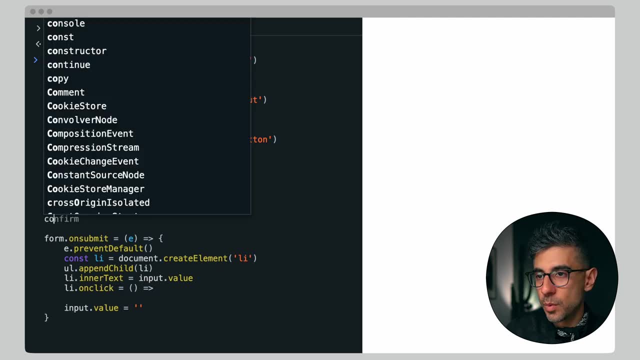 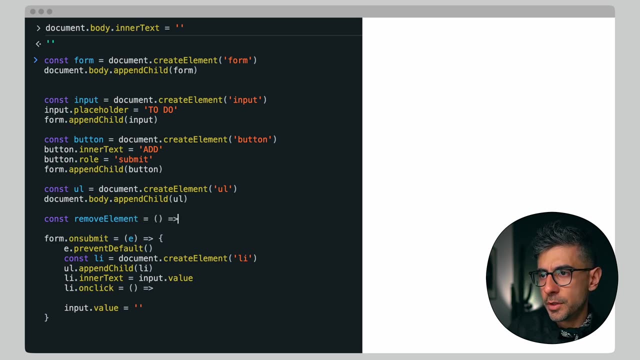 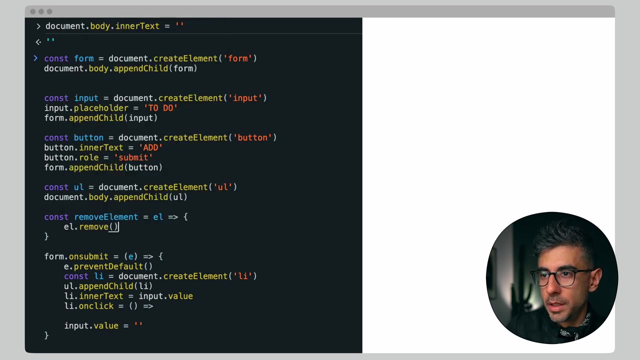 An on click is added to it. slightly better Approach here would be if I just had a reference to this As a function. let's see if this works. const remove element a. I can say equals Function that takes an element L, L that remove. Why is this better? this is better because 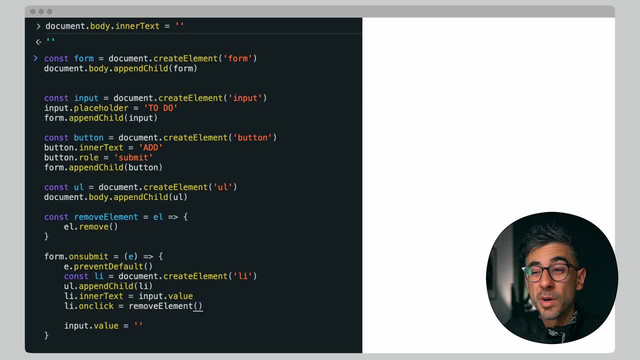 I'm. This is better because We're not creating this function every time for every element. We're just referring to it. It's okay If you have like a few elements on the page. the memory footprint is really what we're worried about here. if you had a giant, 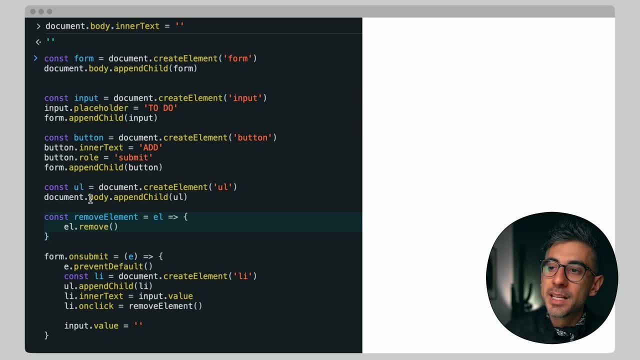 Function and you were creating it at thousands of times. You don't want to do that this way. It's still better practice to do it this way. So there's a lot here that I don't know. Maybe I missed something. Let's see what happens. 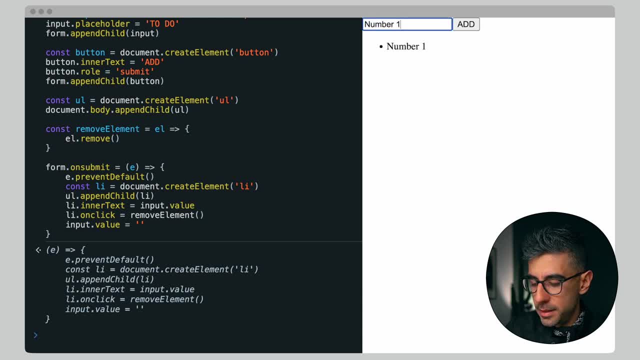 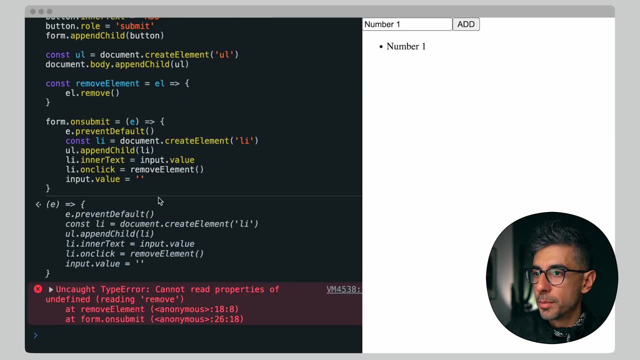 We create it, number one gets added. Oh, we're not clearing the Value. maybe I have some kind of. oh yeah, I do have an error here. Show my errors. cannot property reading. Oh, you know what happened. I am NOT passing the element. 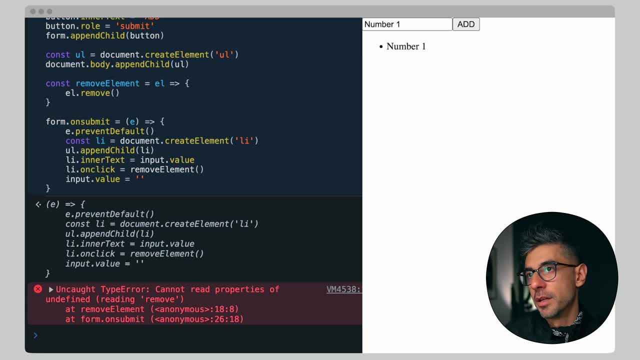 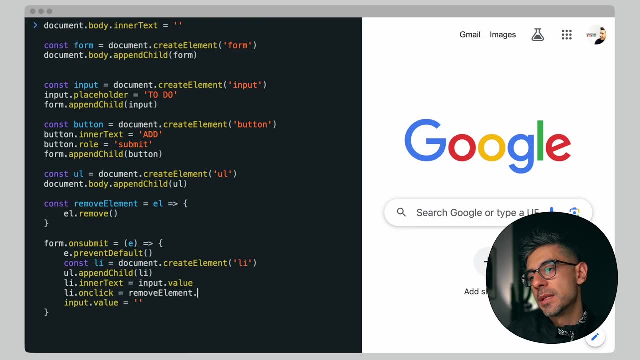 I'm not passing the and the reference to the elements, to the function. So let's do this. We have to do this one more time. Okay, we can do this one more time. a real demo. What we could use is probably function, that's. 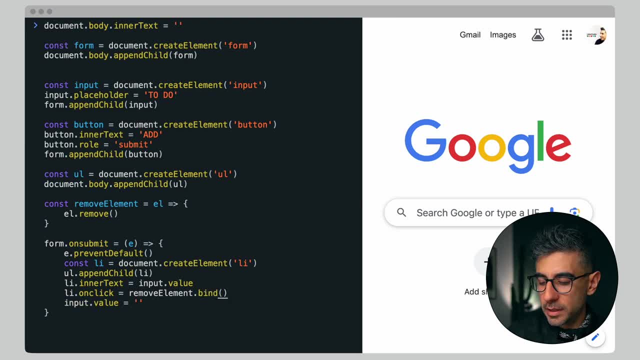 bind Bind. I covered a few episodes ago during the, I think, the prototype episode. What bind takes is The disk keyword, a reference to this. you can bind it to that and then it takes parameters as to what you want to pass There. so I think I can pass a lie in there as a second parameter and it will be this element. 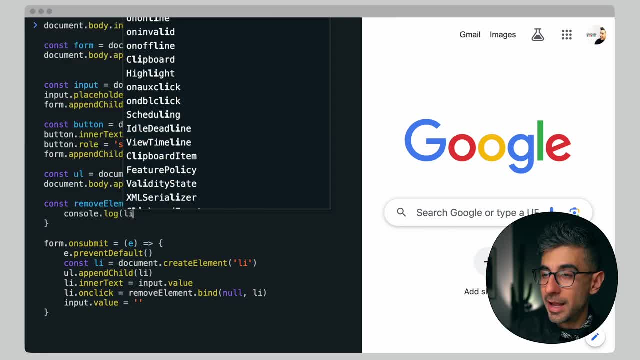 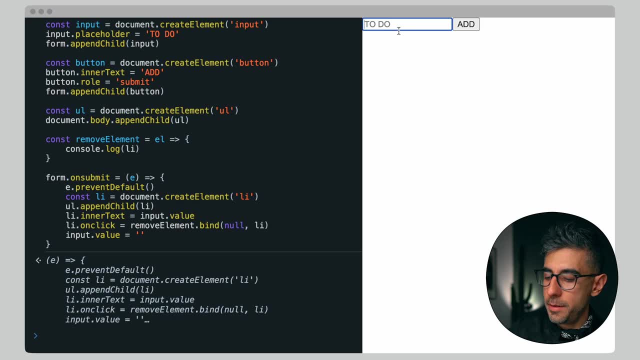 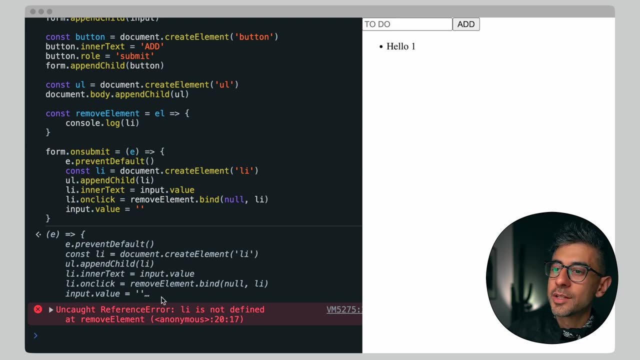 What we can do. you know, we can just do consolelog a lie and see what, see what a lie is. first Let's do that. Okay, Hello one, It gets there. And then, when I click it, a lie is not defined at Dremel, It's called L man. 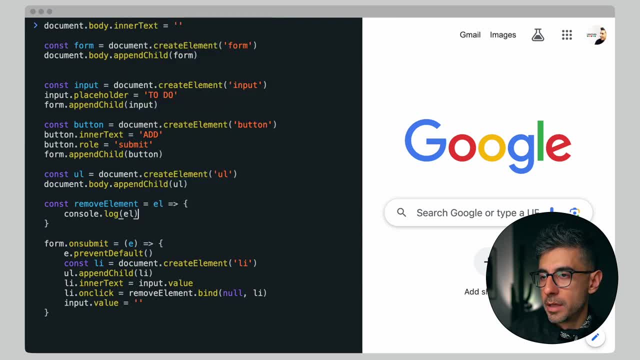 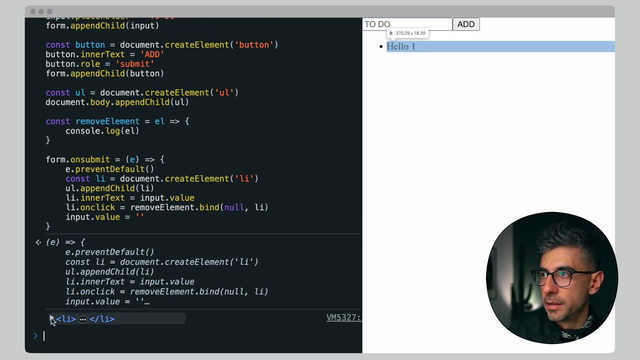 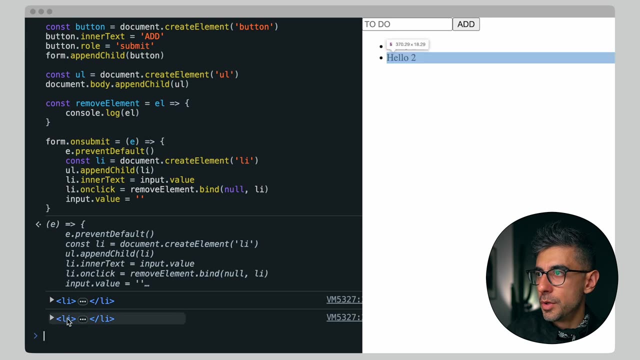 I'm making so many mistakes today. L, Let's do that. and then hello one when I click it. okay, that's my ally, and If I do hello to Click it, that's my hello to all. right, Perfect, So let's redo this for the last time. 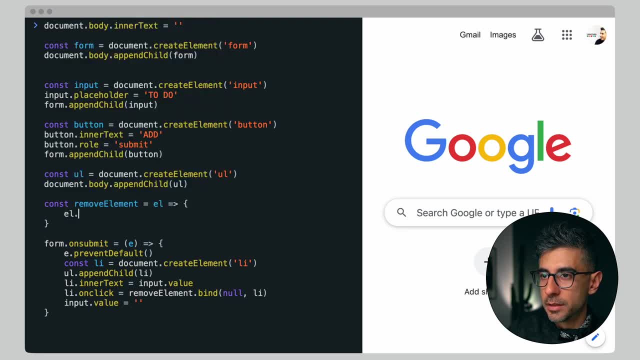 Instead of doing consoledog, I want to say L dots, remove, so remove yourself. Remove the element. I'm passing to it. It's actually very nice. This is kind of a functional way of writing it. It's the next episode and so submit. 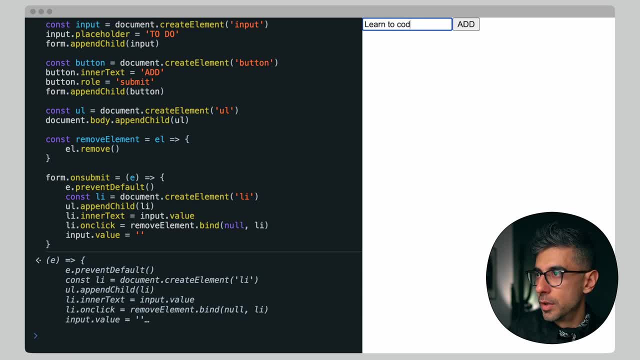 Fantastico. and I can say: learn to code, learn Z Dom. Then I'm gonna get coffee with Ryan Crow. I'm actually a little late. get coffee with Ryan and then afterwards, What am I doing this afternoon? I'm probably gonna be editing this video. edit a video for. 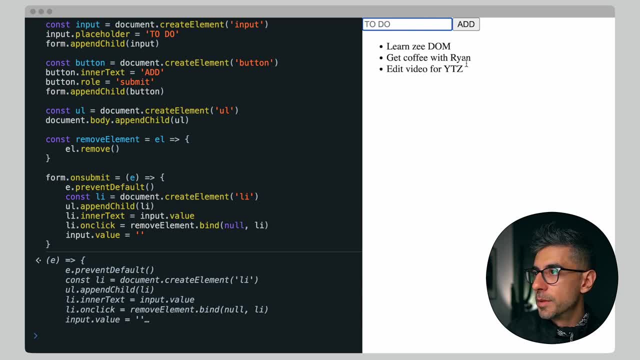 YouTube's. Okay, so if I want to remove them now, click the second one and it goes away. look at that: We're getting rid of the elements dynamically, and so just let's do a ton here and we can just remove whichever We don't want, or as soon as you're done doing your thing. 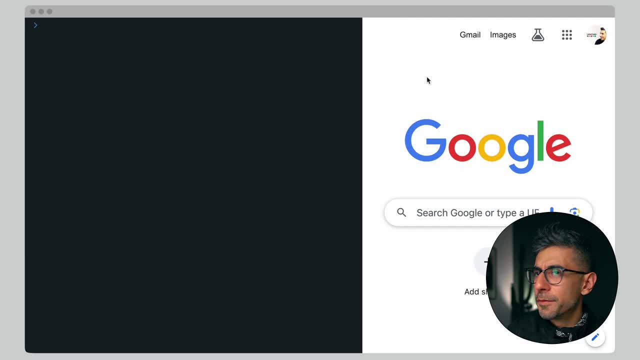 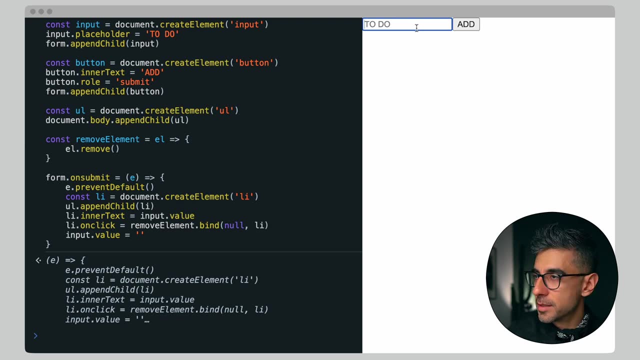 You can just remove them, All right. so that took a few tries, but but we got there. Let me run this one more time. So we have this now. I want to show you a little bit about some of the attributes that you can- you can update. 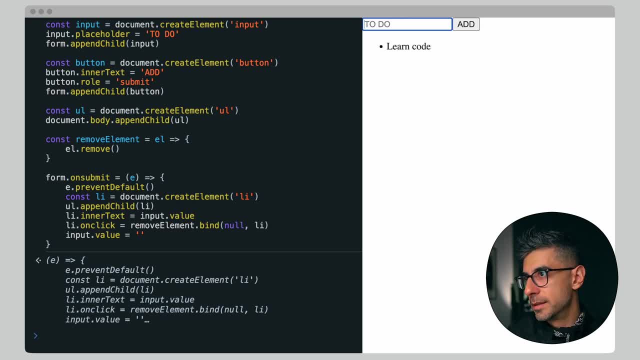 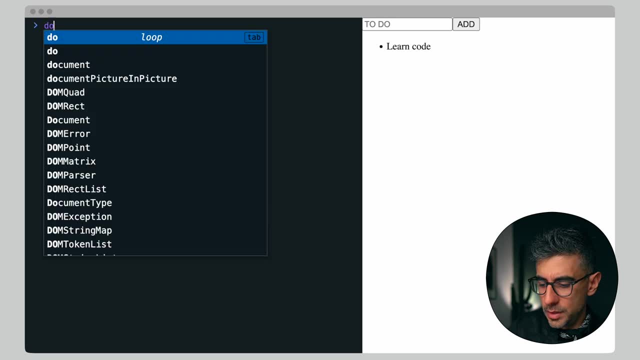 Now we're gonna take this and make it a little bit nicer. So the first thing I want to do is I want to add: Let's see What types of attributes do we have access to so document. Let's pretend we didn't have any CSS here. 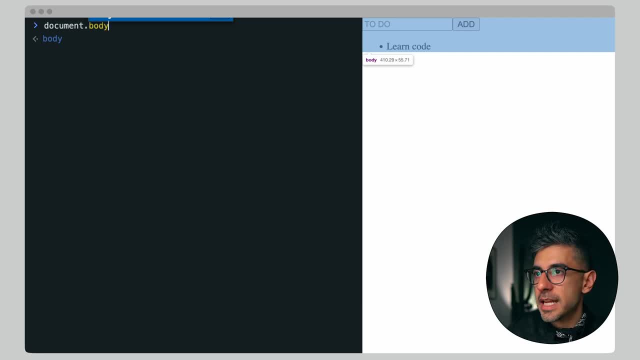 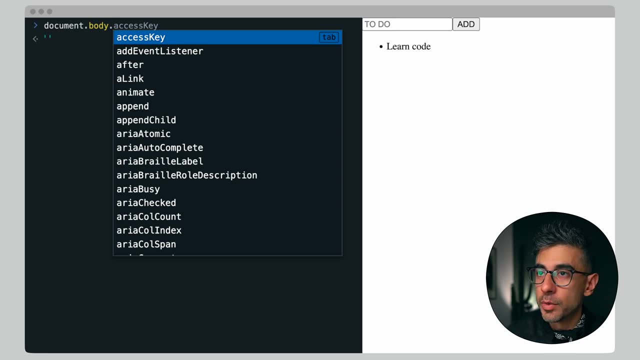 so if we, if we don't have any CSS, and we want to Add, let's say, inline styles, which is not great, But it's a way of adding attributes, so and it's, it's really really visible- a demo as well, So I want to do that document, that body. What did it have? 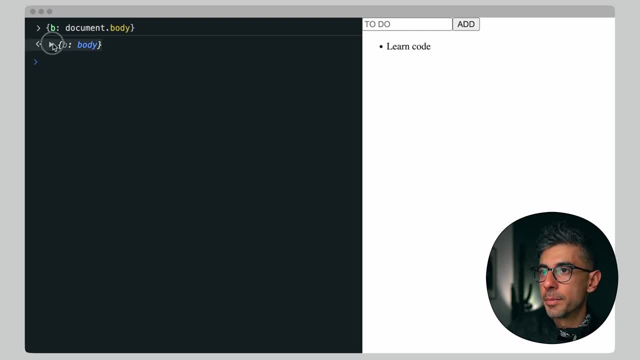 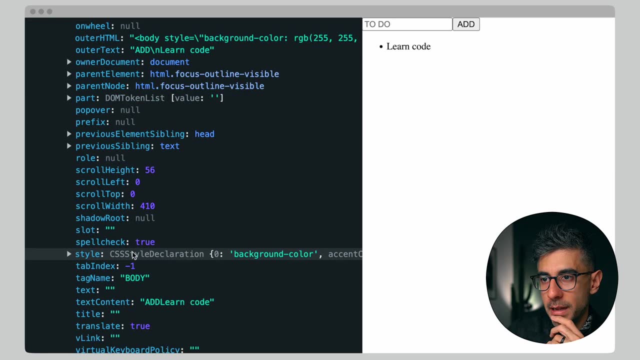 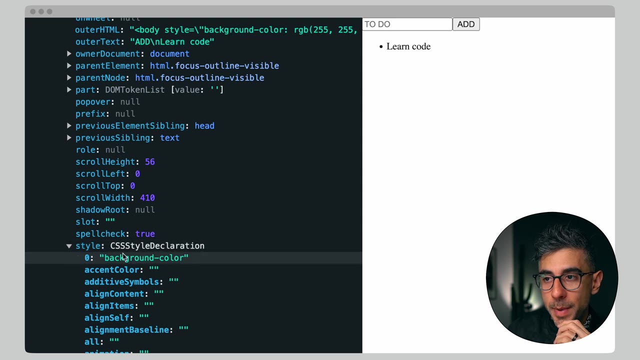 as any sort of Styling property. So if I go into this again, I go all the way down to Wow, there's so much it has to paginate it. style style is a property that every HTML node has, So it has background color. Well, that's not at this. animation stuff There is, there we go: background color. 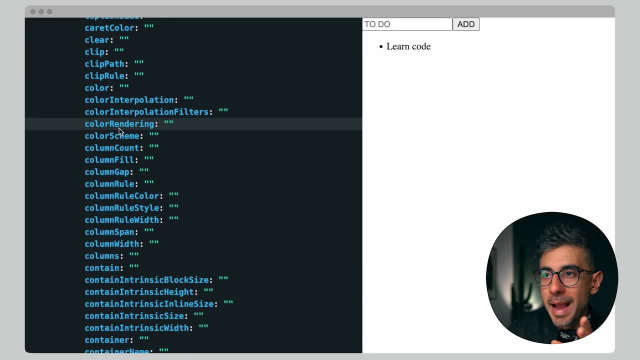 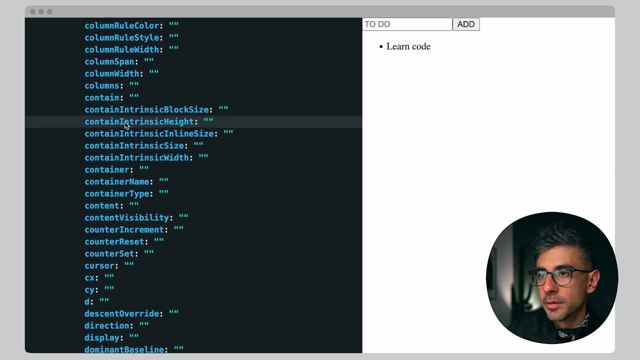 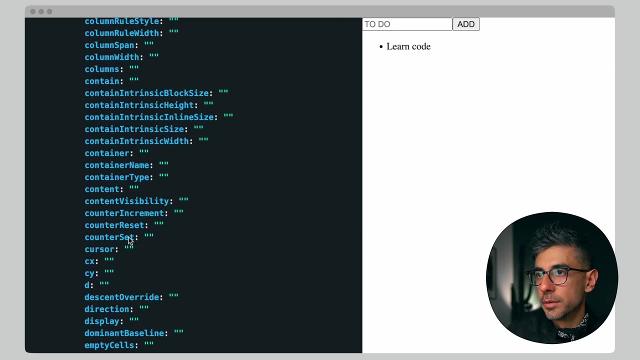 background image. any CSS property you can imagine here is. You have access to it. except you can't do Kebab case or or snake case. It has to be camel case, the way you see here, So something like a background color. it would have to be camel case. What do I mean by that? 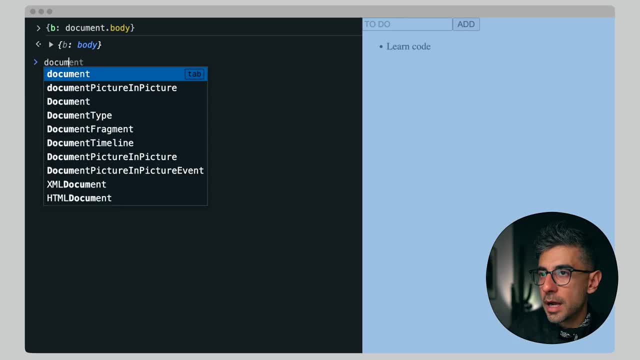 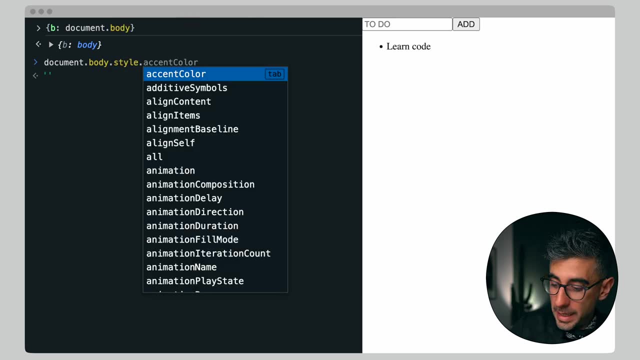 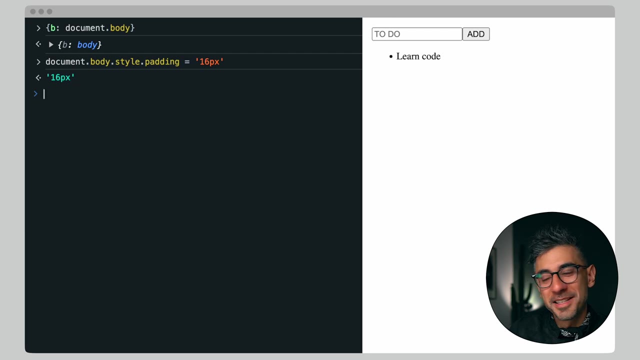 Let's, let's try a few things here So we can say: document that body, Stud, style, dot. What do I want to do? a padding- Let's add some padding here- equals 16 pixels. Nice, did you pay attention to this? Great, then I want to do: 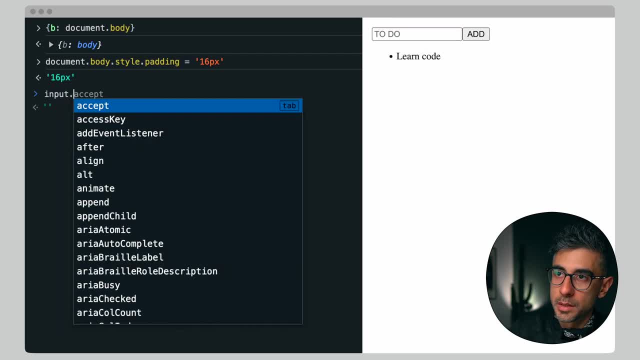 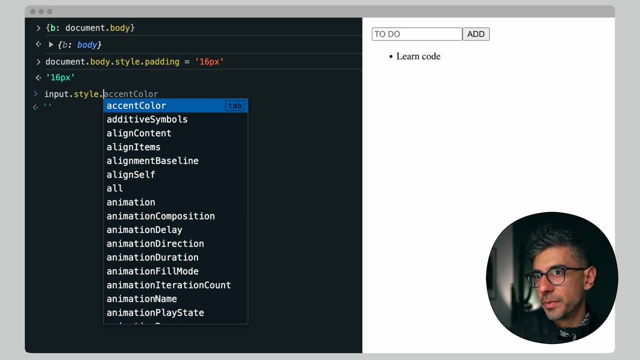 Can I add stuff to other elements? inputs, dot style. Sure, and the reason why we have access to input is because I just Created the element. I just got rid of my console, but I do have a reference to input. We probably don't want to do this after you created it. You want to do it kind of as the same process. 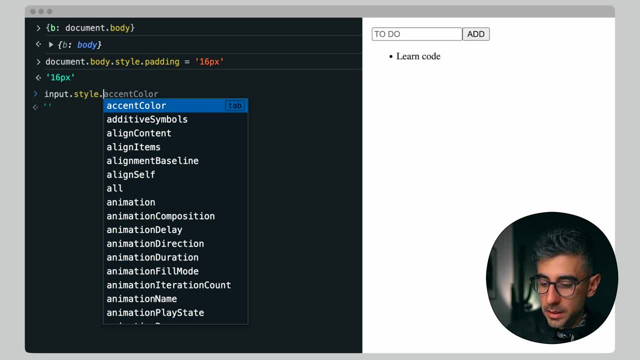 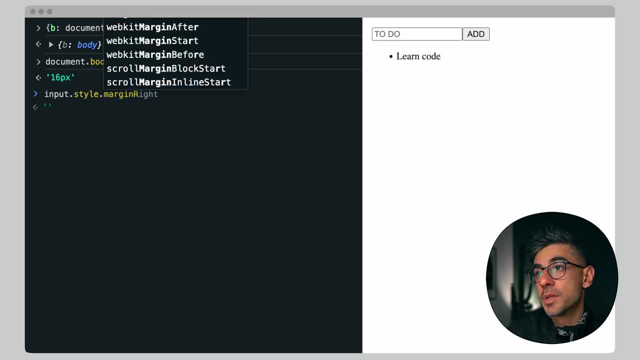 But I can say: input that style dots. I Don't like the fact that it's touching the add button. I can say: margin right, And this is what I was talking about, where I said things need to be camel case as opposed to CSS. You can't do that. 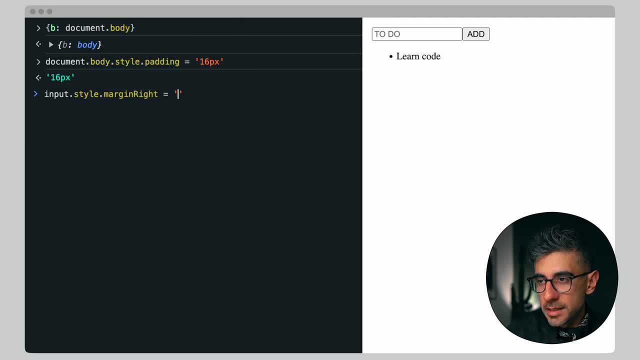 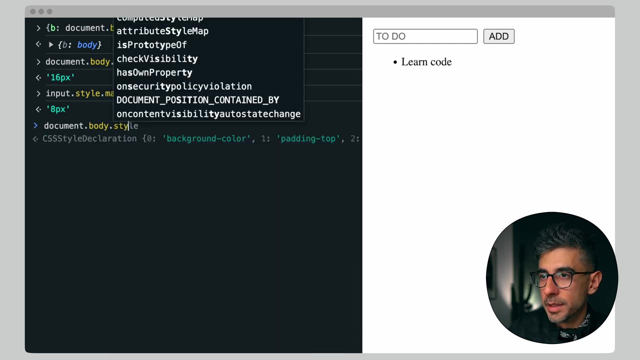 Because that's not allowed in JavaScript. Let's give it eight pixels. Let's stick with a Similar. there we go. similar kind of styling. you can do anything you want. you can change all the colors if you want it. We can make this super ugly, but it's just for the sake of showing it to you. background color equals red. Ah. 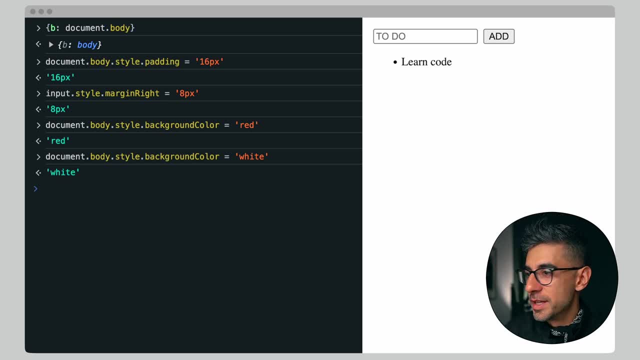 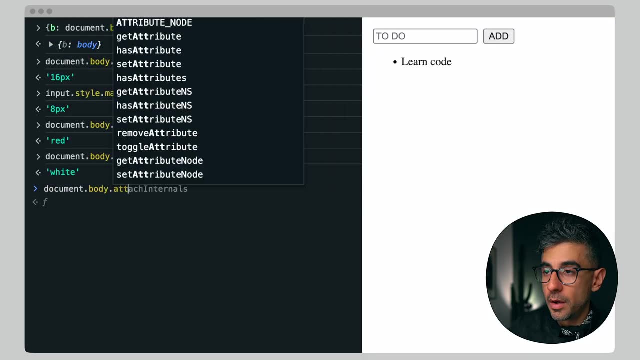 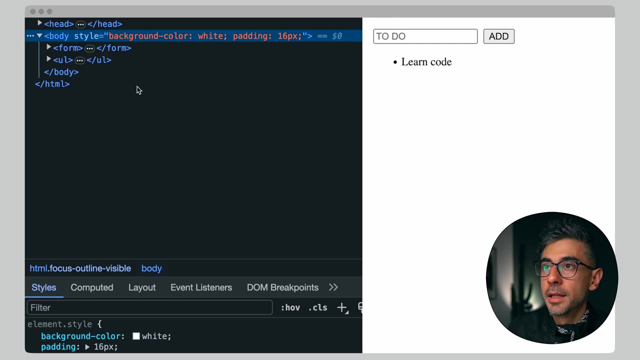 Back to white, back back to a non so abrasive red. So that's pretty cool. The other thing you can do is document that body, that attributes all together. It shows you all the things that it has on it. So we added a style Attribute there which is this: right, So it. I have access to those. I can say All right. 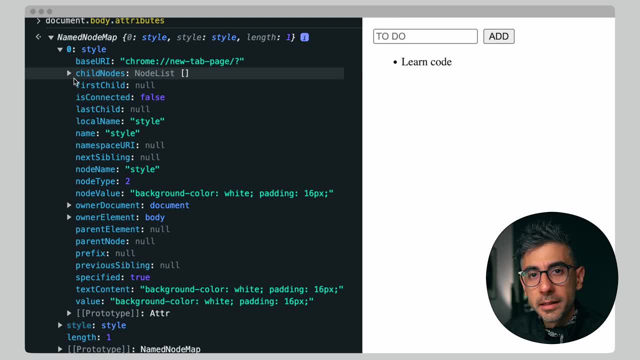 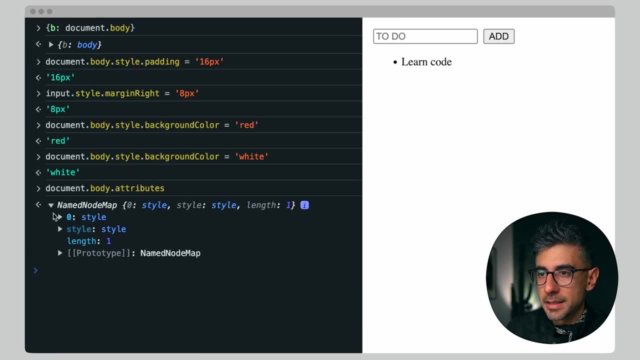 tell me what other things are in there. I can read my attributes, like my IDs or classes or anything else that's on there I have access to. I can read those so. So let's create another attributes. so style It does the job for us, where it creates the attribute and adds it. 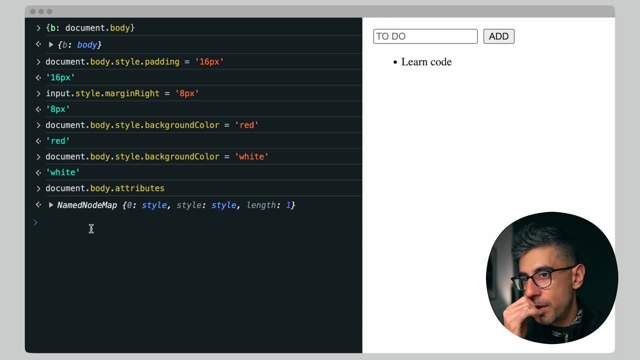 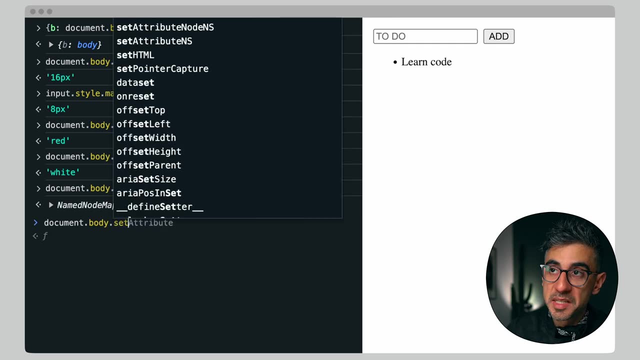 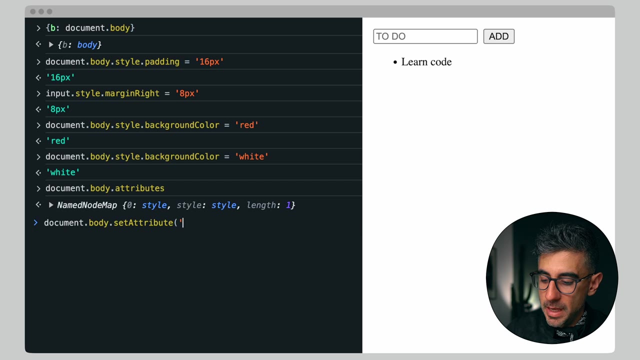 What if I want to add a ID to this or a class? we probably don't want to do an ID, So let's do a class. Document that body, What do you think it is, set, Attribute and what does it take? a name and a value. the name is: I want to do a class and 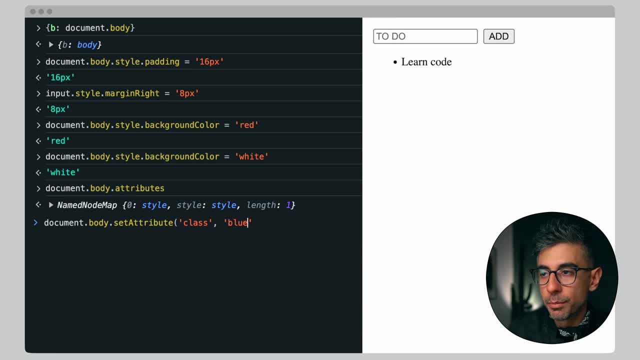 the value is Blue. it's not gonna turn it blue because it's just a class. but let's say you had a CSS style sheet where you had a dot class and You had the background be blue. You can apply the class to the element and Then it would just the styles would apply. 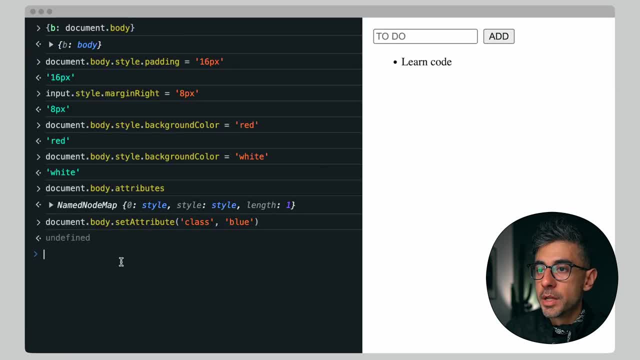 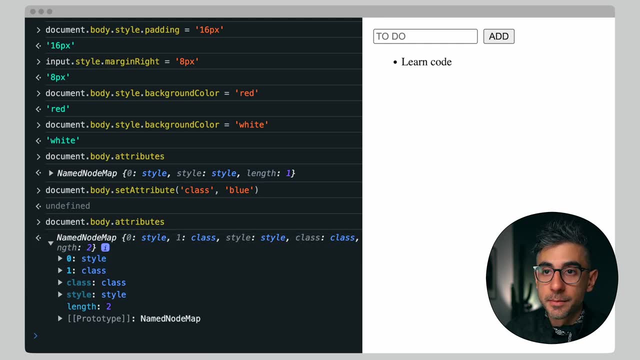 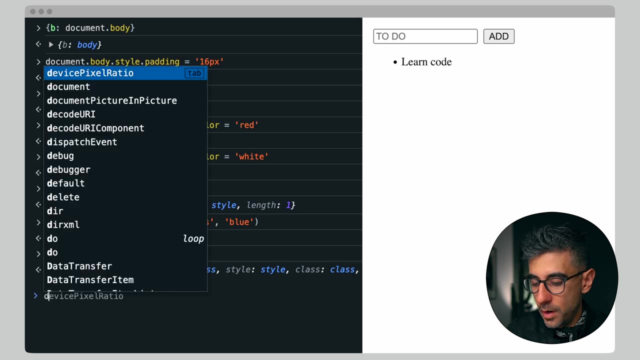 So now the class blue is also on my body, so if I do Attributes instead of one, I c2.. I see style and I see class. Cool, So Let's go back to the read operation. We're almost through here. The way we read so far is documentbody. 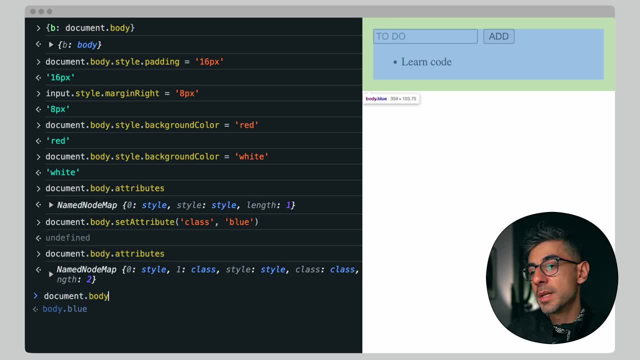 and that's not great, right? We don't want to go through the body every time We want to say document. There are different ways to query the DOM, so to speak, Get coffee. so I want to have multiple things here. 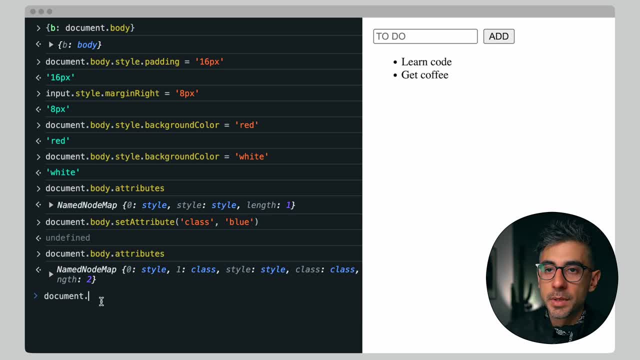 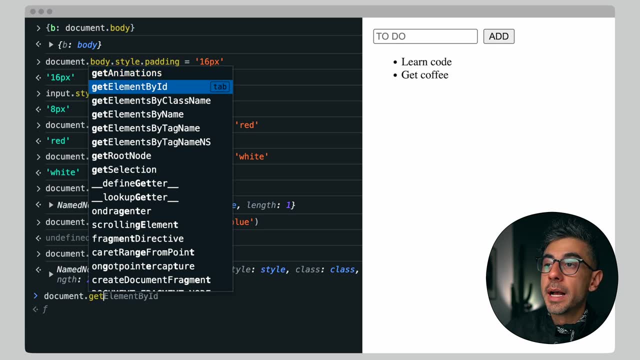 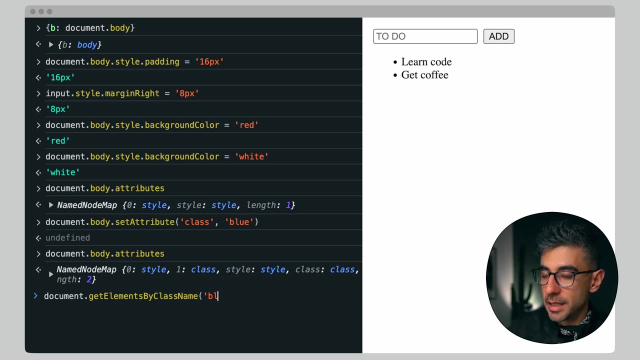 So how do we get all the? how do we query the DOM? using the DOM API? We can say: document there's a few things here. If I write get there's a bunch here, Get element by class name, okay, And then obviously we have to pass it a class name. 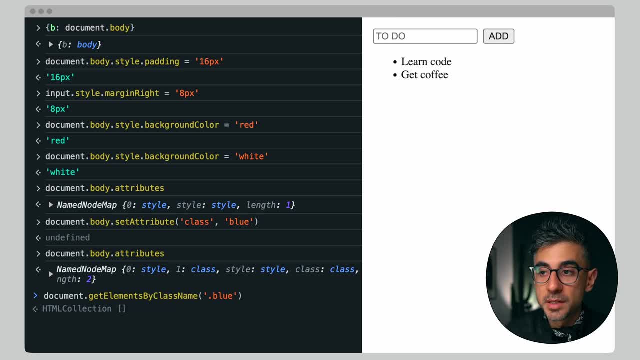 Let's say blue. Remember you don't have to put the dot here, because you're already saying you're specifying that you want to get it by class. So it's not a CSS selector, it's just a class name. If I do that, it says: well, it gives me an HTML collection. 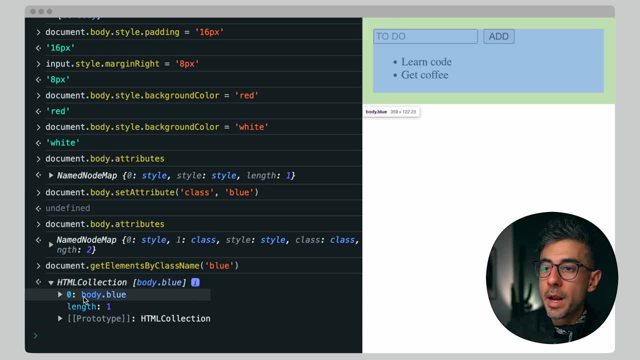 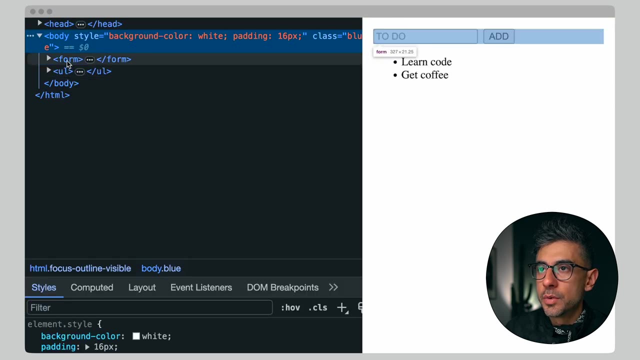 which is effectively an array, And it says: you have one element in that array, the length is one and that is the body And that's the element where I dynamically, manually, using code, I added this class to. In fact, if I go to the form and do this, 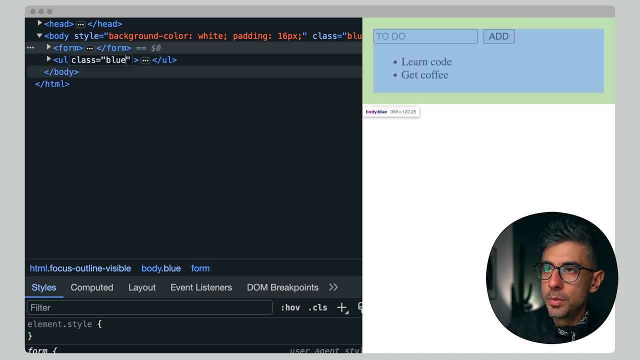 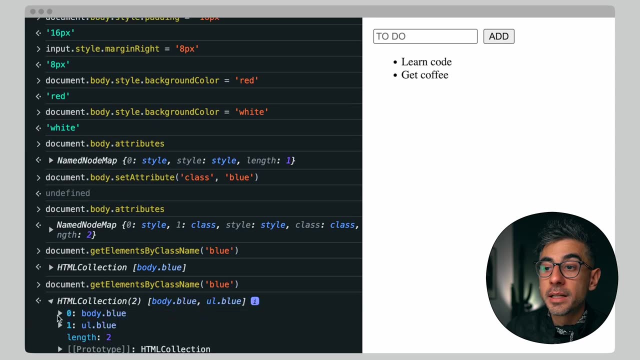 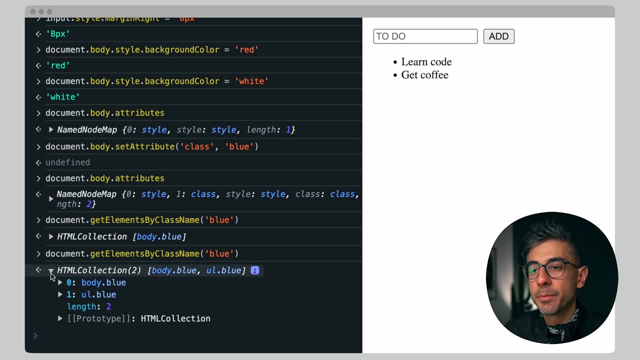 add attributes: class blue. Obviously, this is just for testing purposes, just to see this work. Now my collection has two: It has the body and the UL. So when you run your query, it at that particular moment goes through the DOM. 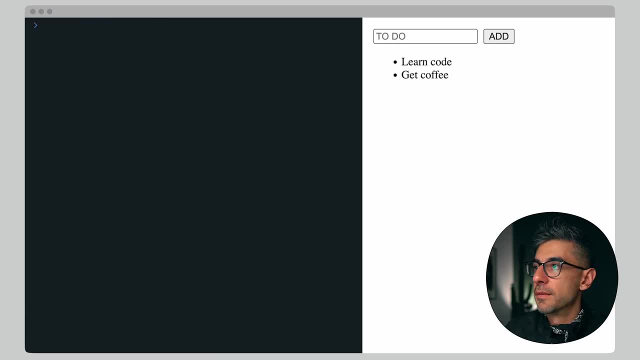 finds all the things that you need, that you queried for, and it gives them to you. So what else can we do? Get elements- This is get multiple, get elements by class, because you're allowed to have multiple things with the same class. 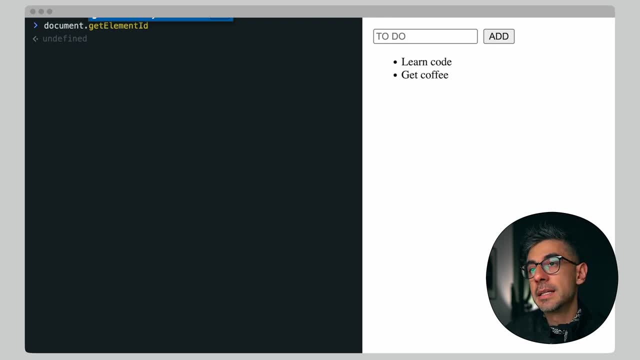 But you can also say get elements by ID. I don't have anything with any IDs in there, so this is probably useless for me right now. Get elements. Get elements by tag name. We have two LIs. Let's see if it gives me the two of them. 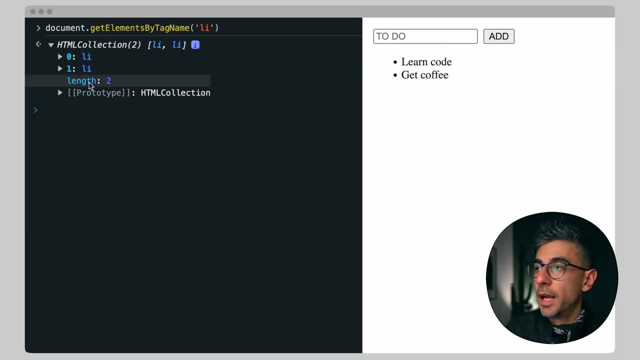 Yeah, perfect. So this way I can. I don't know what's a good use case for this. You can have a button on the bottom of the screen or at the top or whatever, to say remove the latest or remove the oldest right. 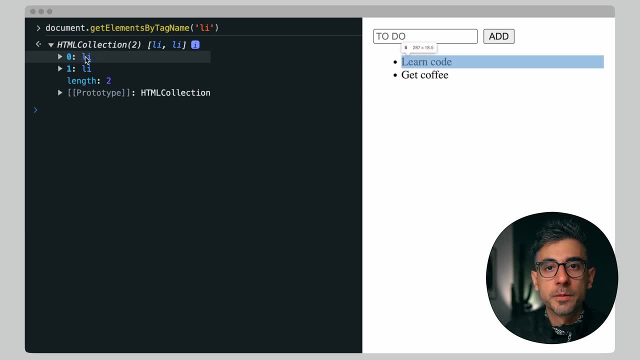 You can get the list of LIs and grab the first one from the list or the last one, whichever you wanna do. So it gives you a lot of control, as you can see, But the most powerful of all is document dot. it's not actually get it's query. 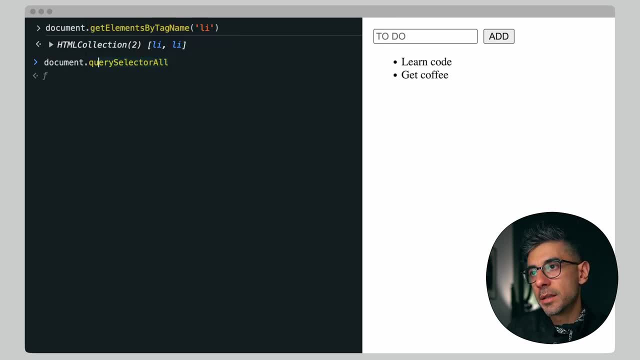 Query selector and selector, all So query selector: what it does is it actually takes a CSS selector So I can say dot blue. So now I have to put the dot there And it gives me the body. but wait a minute. 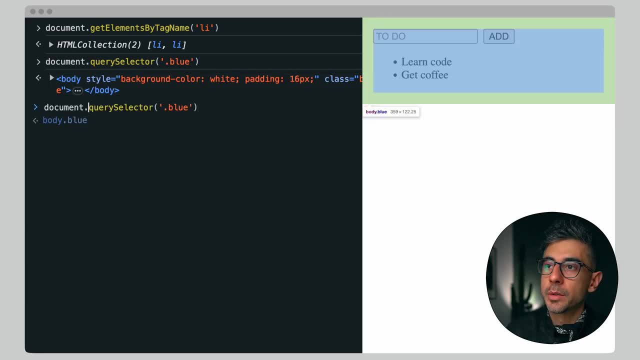 didn't we have two? Yes, we did have two. and that's where query selector all comes into play. You can say: body and the UL, Both of these guys return. So those are. let's do the Li as well. 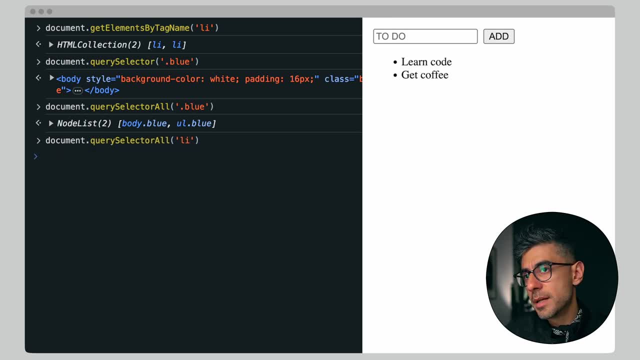 So it doesn't have to be a class, it can be element type. So now it's a node list of two Li one and two. So it's an extremely powerful way of basically scraping what's on the DOM. A lot of the sites that do web scraping. 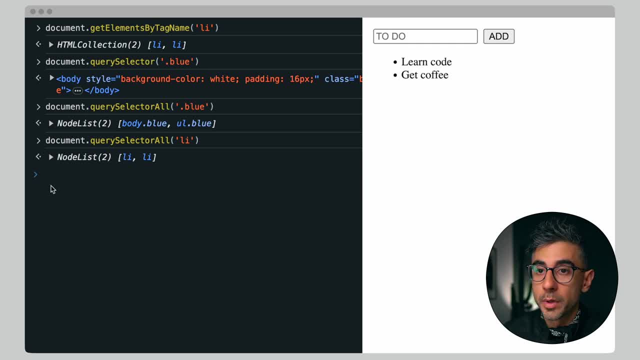 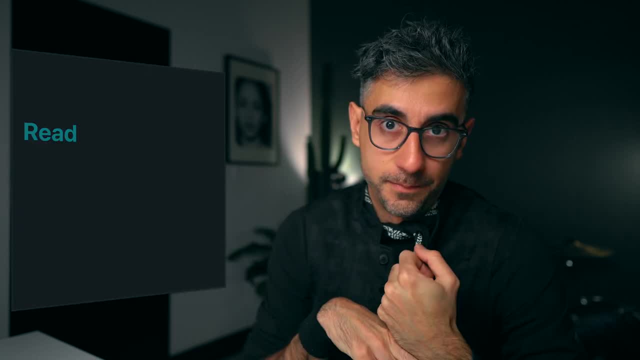 if you've heard the term, they have to use some of this to query the DOM. Okay, so here is everything that we looked at today. We can read elements, We can read their attributes. Within their attributes, we can get their styles. 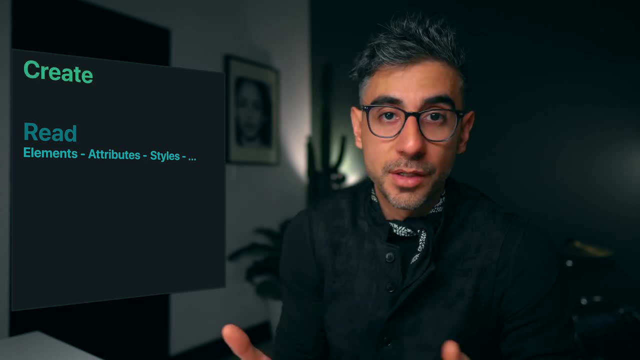 their IDs and classes. We also saw that we can create new attributes and add it to any element. We can create new elements altogether using a type of element, a tag name, and we can add them to the DOM, to any particular parent's. 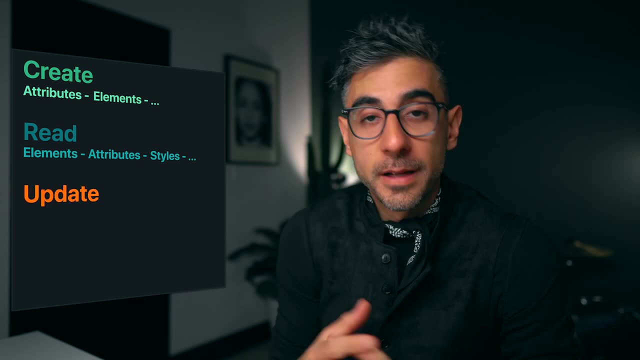 element, So we can create any element that we want. Then we saw that we can also add events handlers, including click and a whole host of other events that I didn't go through today, but that's what MDN and documentation is for. 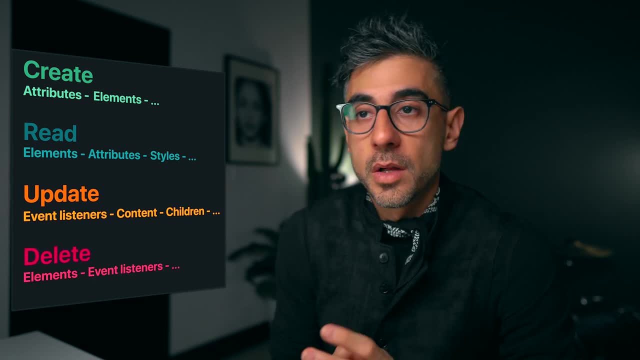 And we also saw that we can remove elements from the DOM as long as we have a reference to that element, And that, my friends, barely covers- I don't know 10% of what the DOM API can do. I mean, it's what's capable of. 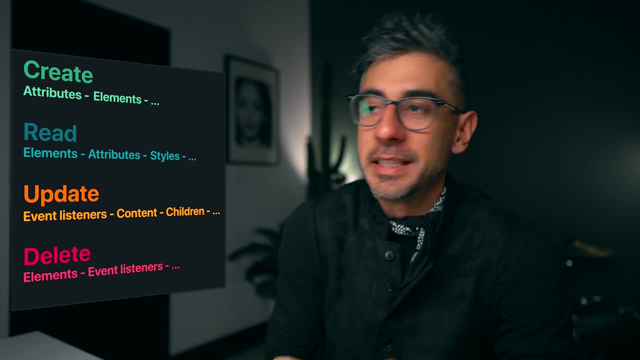 There's so much more you can do. My goal is not to show you everything that this API can do. My goal is to show you how powerful this is and that you can probably do whatever you think you need to do with the DOM itself. 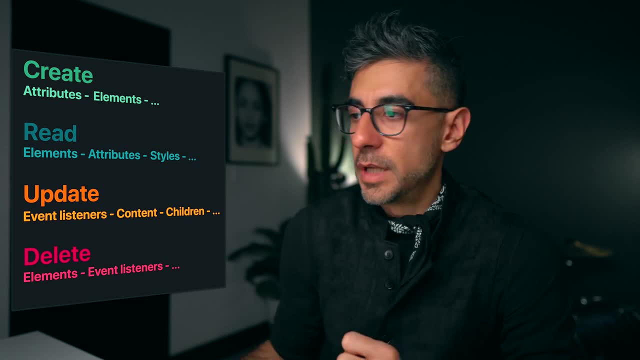 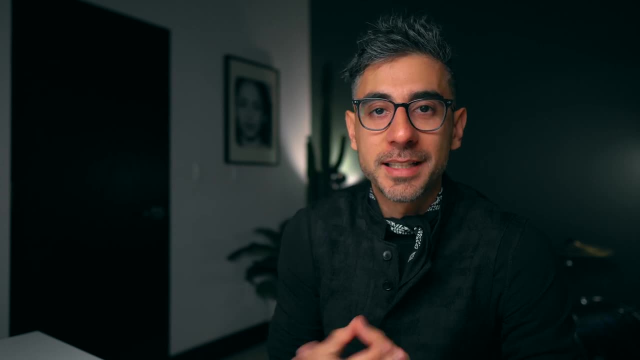 with the API itself, And the best place to look for documentation is our good friend MDN. Hopefully that gave you an idea of how crazy powerful this stuff is and what React and Angular and all your favorite tools are doing under the hood, or jQuery for old like me. 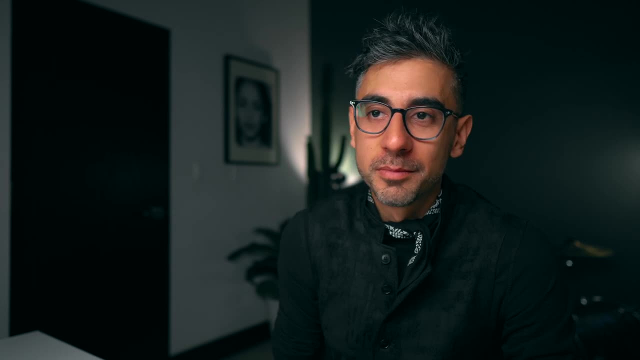 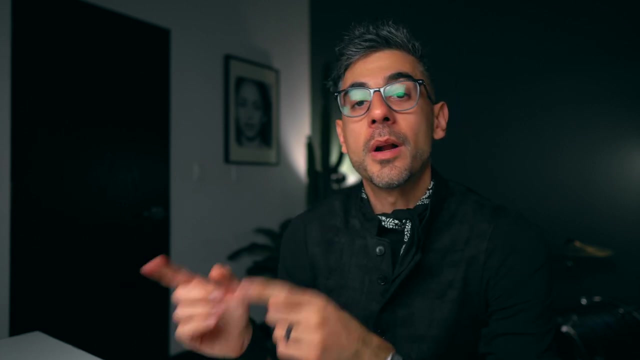 It's not magic, It's just they're just using the pure browser API. But obviously the benefit of those things is that you have to write a lot less code. I wrote a lot of code here today, So I'm gonna put all this code up on GitHub. 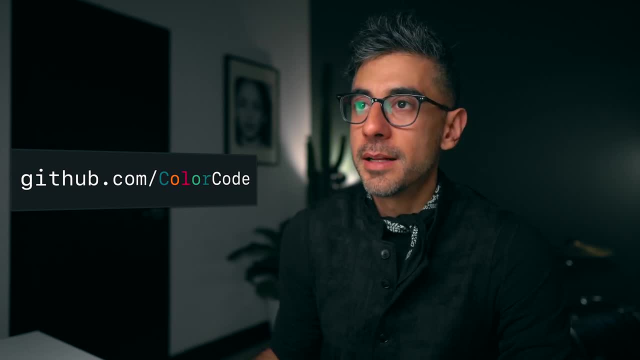 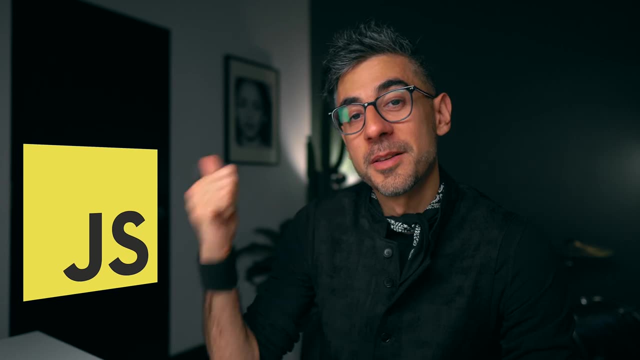 in case you wanna look at it. But again, the best place to look is MDN, and that's it. Now, what should be the next episode? I'm so glad you asked. I actually already told you, So this has been episode 15. 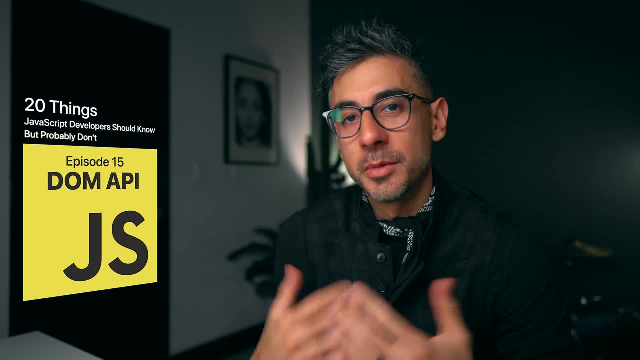 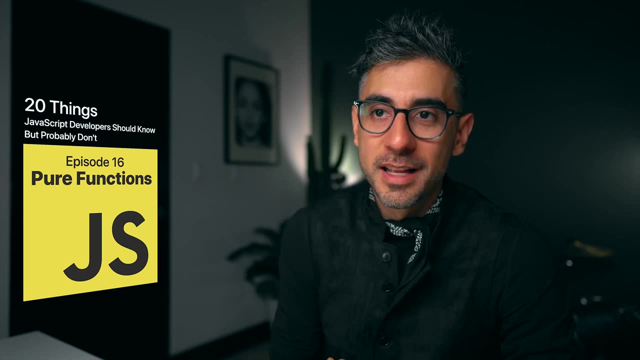 of 20 things JavaScript developers should know, but probably don't. I'm glad to be back. Next episode will be Pure Functions, episode 16.. Be sure to tune in. It's an episode. It's an important concept in modern JavaScript. 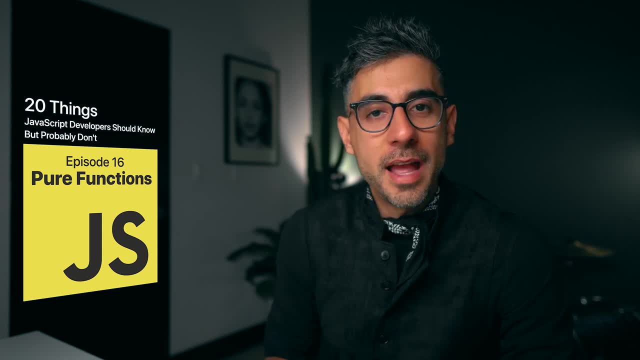 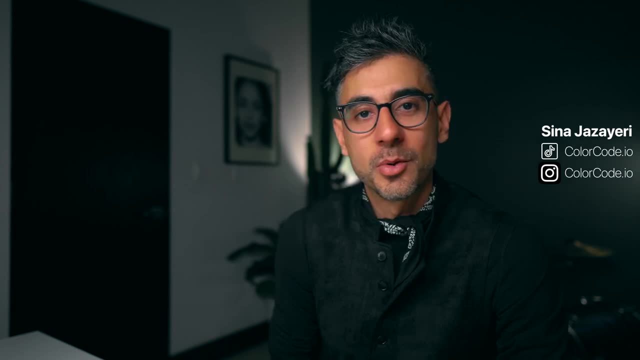 This is a fundamental piece to functional programming. I will see you then, and come find me on Instagram for personal posts and one minute shorts of all the same videos I'm doing here. All right, good to see you. I promise it won't be another six months. 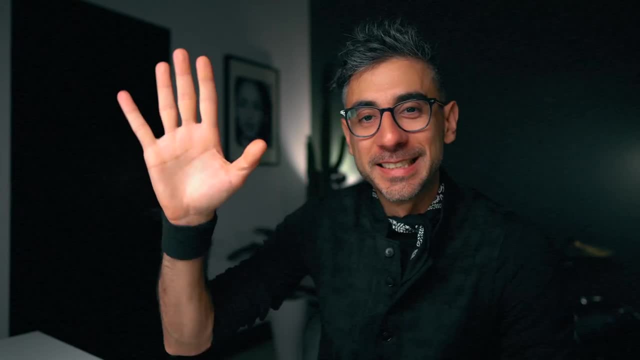 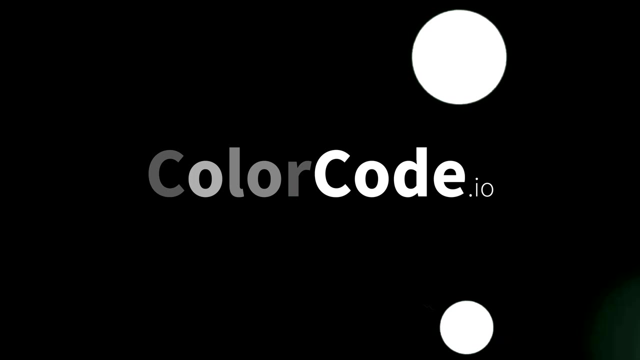 before the next video: It'll probably drop in a couple of weeks. All right, See you next time. Bye.